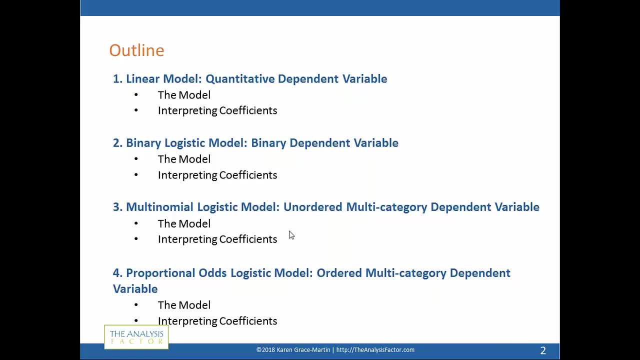 there are more similarities than there are differences, So we're going to talk about how they're the same, how they're all the same, how they're all the same, How they're a bit different and why that difference is something you can absolutely wrap your head around. 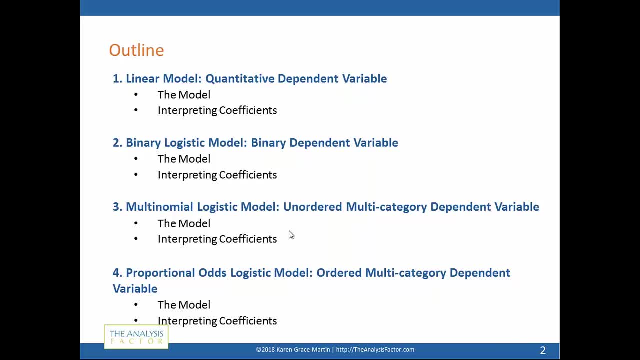 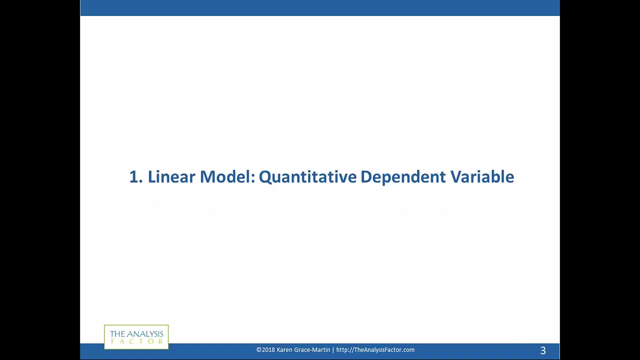 even though they can look absolutely strange at first. So we will go through each of these three types of logistic models: The case for binary dependent variables, for unordered multi-category dependent variables and for ordered multi-category. Okay, so let's start with the linear model. 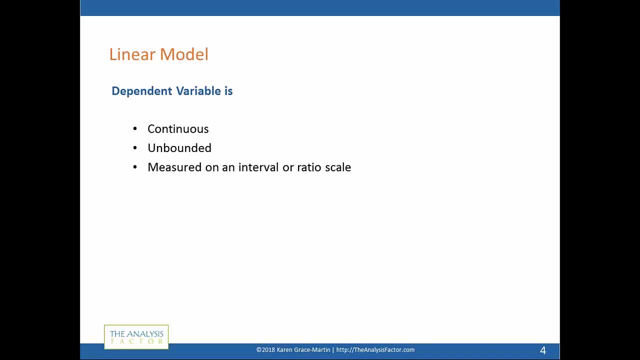 Okay, there's a lot of confusion about this, but linear models work when we have a set of predictors and we want to see how well or to what extent those predictors are related to, or help us predict, a dependent variable that is continuous. okay. 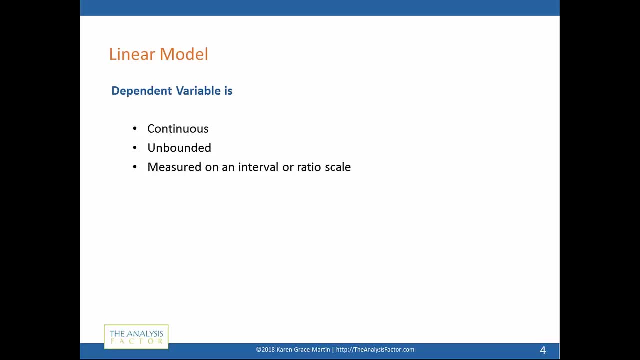 So, again, we should have a set of predictors and a set of predictors. So the first one is that we have to have, technically, we should have- truly continuous values unbounded. so again, no boundaries above which or below which the values cannot go. 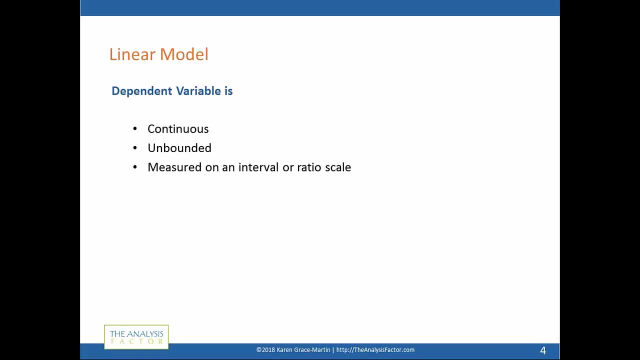 So, for example, percentages are a great example of a variable that is continuous. so we may want to fit a linear model, but we often have trouble with meeting normality assumptions and particularly if the data are pushed up against those boundaries. this can. 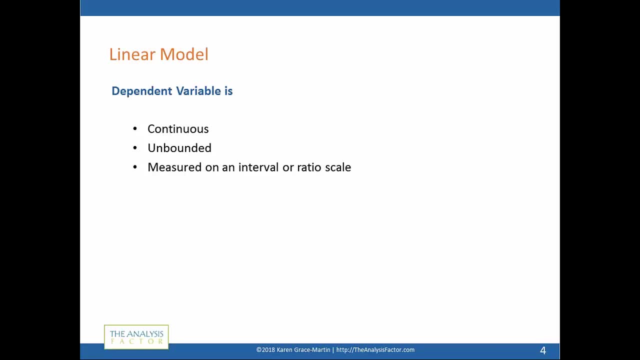 become a problem. if they're all in the middle, we often can get away with it, but if they're at the boundaries it becomes a problem. and then, third, measured on an interval or ratio scale. so you'll notice I'm not saying that the dependent variable has to be normally distributed. the true assumption about normality is: 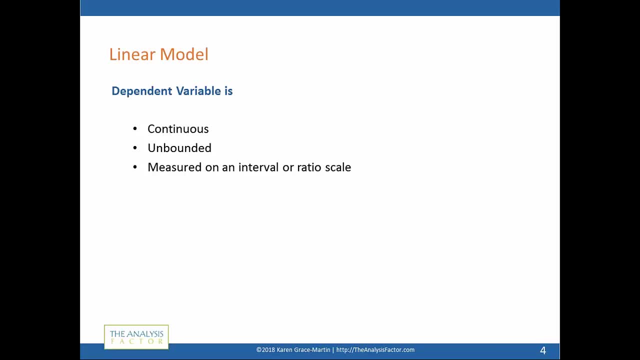 about the residuals. but if these three conditions are not met, it's usually impossible to get- I shouldn't say impossible, but it can be very difficult to achieve- normality of residuals if we don't have all three of these conditions met. okay, I'm sure you've all seen this model before, but let's walk through it. 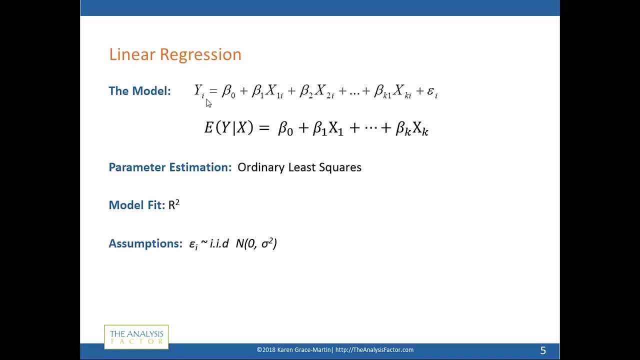 just a bit. we have an outcome variable y. it's measured on each subject, which is why it has an i subscript, i subscript. we have the intercept, which, of course, the intercept tells us it anchors the regression line right, how it tells us about the height of the line. we have the effect of each predictor, x, so we have a. 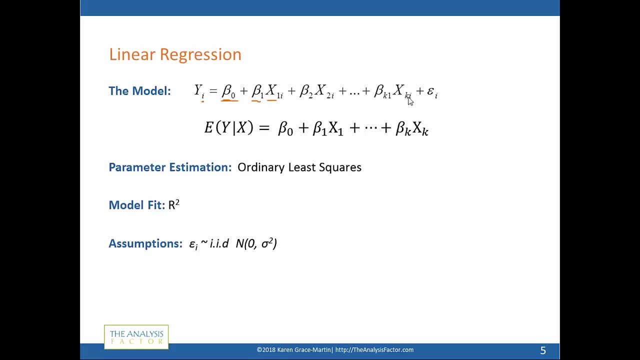 set of predictors: x1, x2, all the way up to xk. each x has an i subscript as well, because each subject has a value of x. but the beta ones, they are a summary measure, they're a parameter of the model: beta 1, beta 2 and so on. and 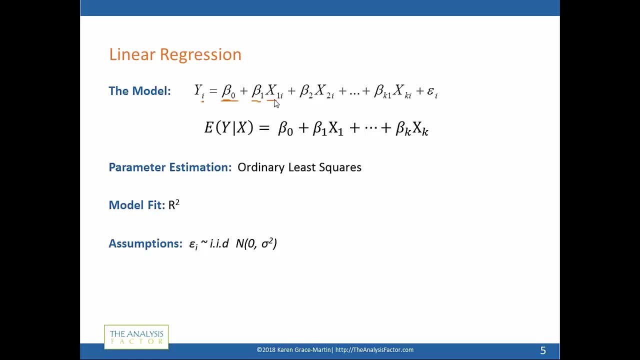 each one tells us the effect of the corresponding X on that Y, on average right across all of our subjects. so to what extent does X affect Y? you know it's a good question. we're not going to go into that in detail, but let's start with the model. the model today is going to direct us in the form of. 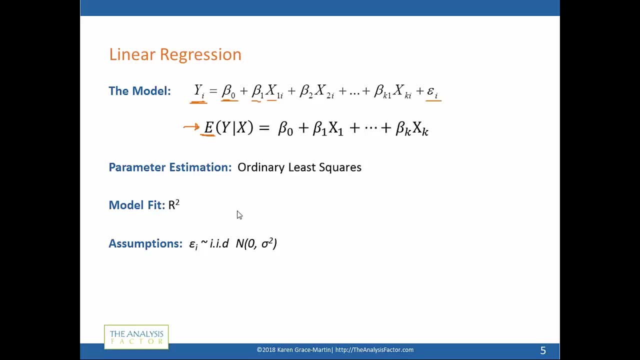 characteristic of Y and its functions. and its functions are going to be represented as variables and not as Wild all the way up to Z. so we're going to see that as a function. as we draw this, we're going to see that the function that we're going to give to Y and its functions are going to be represented as: 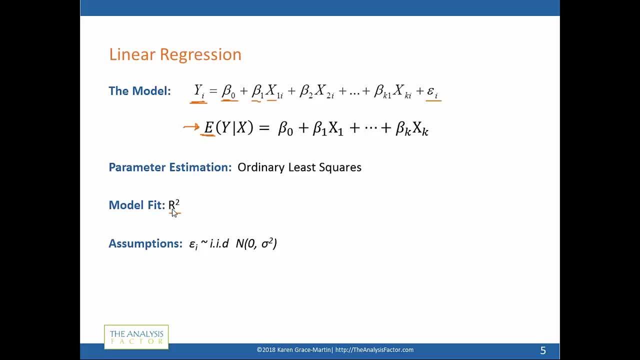 In addition to, you know, giving us an indication of model fit. it's very nicely intuitive. It has a nice interpretation of the percent of variance in y in our outcome variable. that can be explained by the axis. And, of course, here's our assumption. 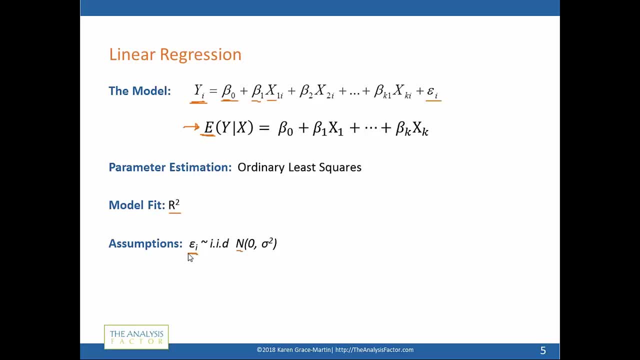 This is where normality comes. in Our error terms, our residuals are distributed, as tilde means distributed, as they are independent and identically distributed. That's iid. So they're independent of each other, but they all come from the same. 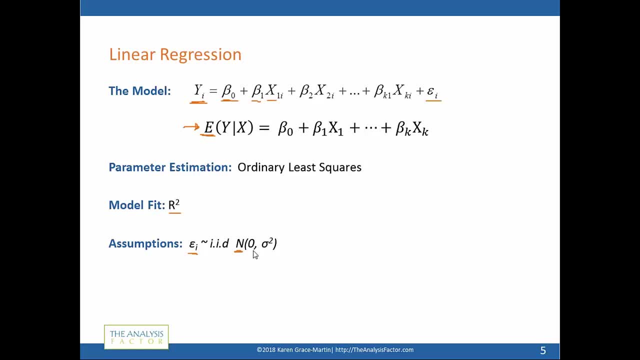 they're all distributed from the same normal distribution with a mean of zero and a variance of sigma squared. Okay, so we don't have some residuals coming from a distribution with one variance and other residuals coming from a different distribution with a different variance. They're all coming from the same. 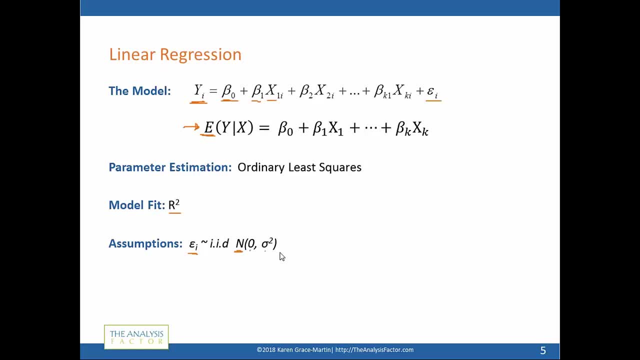 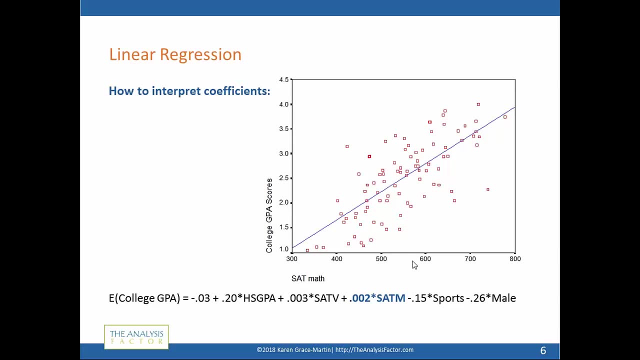 They're all coming from the same population, Okay, and this is, of course, what it looks like. And let's talk about this example we're going to use and how to interpret coefficients. So I just drew the simplest model. I will start off by saying these are not real data. 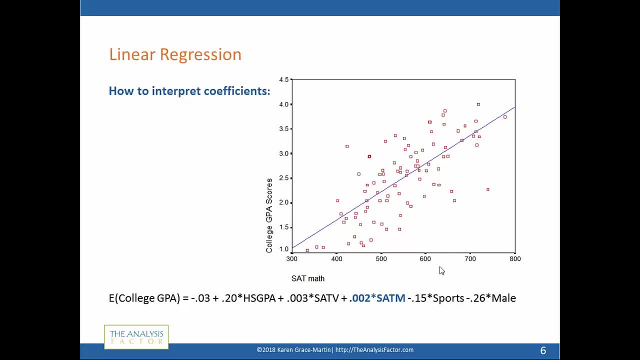 Usually, if you've been in any of my workshops, you know I'm actually pretty picky about always using real data. But here I'm cutting corners a little bit, because it's just so nice to see when you have, when we can really illustrate the point here. 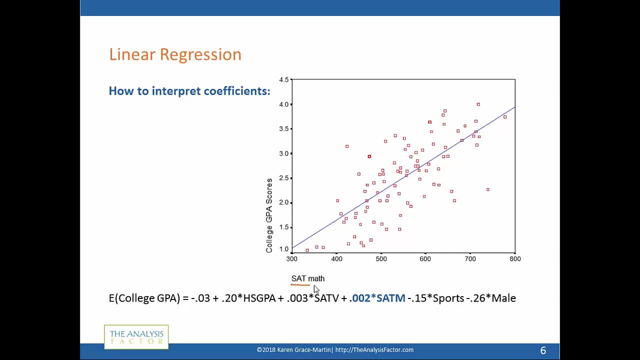 So what we've done here is we can see on the x-axis we have SAT math scores and here on the y-axis we have college GPA scores. Okay, so what we're trying to do is maybe we are admissions officers at a college and we have applicants. 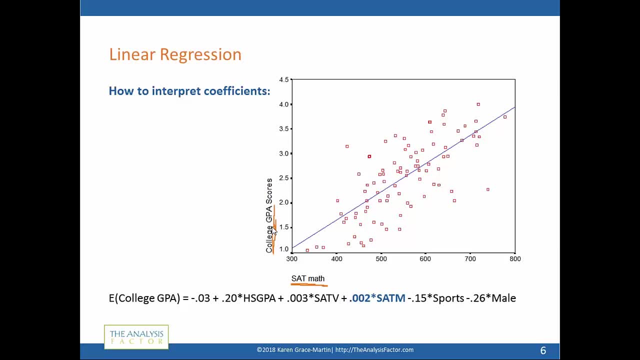 and we're trying to see if among our current students. how did certain information we had about these students from their application, like their high school GPA, their SAT verbal and math, whether or not they played a sport and whether or not they're male or female? 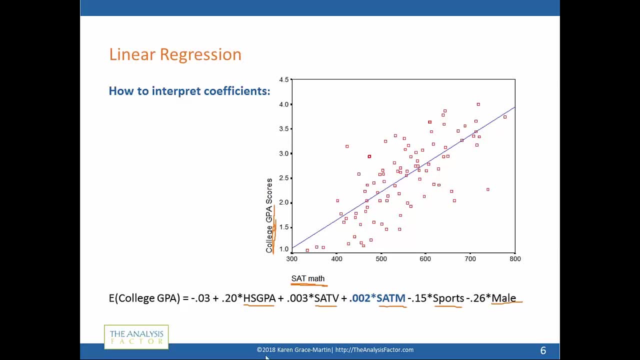 does that predict their GPA? Okay now, both high school and college GPA are on a zero to four scale, but SAT verbal and math are each on a 200 minimum to 800 maximum scale. If you are not familiar with the SAT, they are standardized tests and there's a 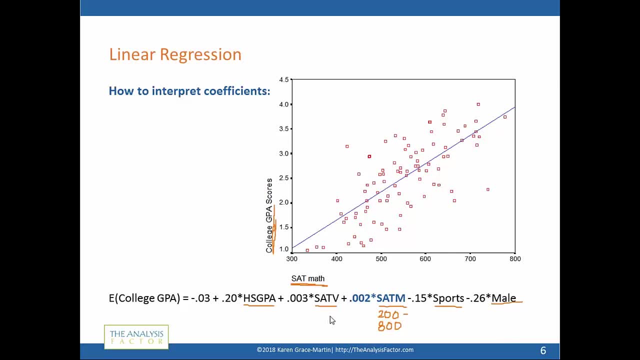 verbal section- it's now called critical reading and writing- and there's a math section, and you get two scores, each of which ranges from 200 to 800.. So a one point difference is very small. Okay, so we can interpret this point: zero, zero, two effect as: 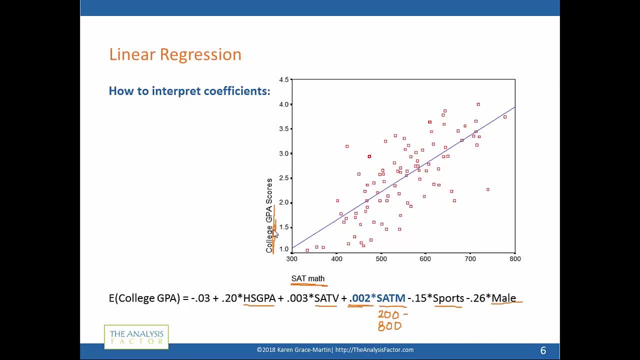 the average increase in college GPA for a one unit increase in SAT math. Now, a one unit increase, as I said, is pretty small but we can just change that. We can move our decimal over like that to get a 0.2 and say: 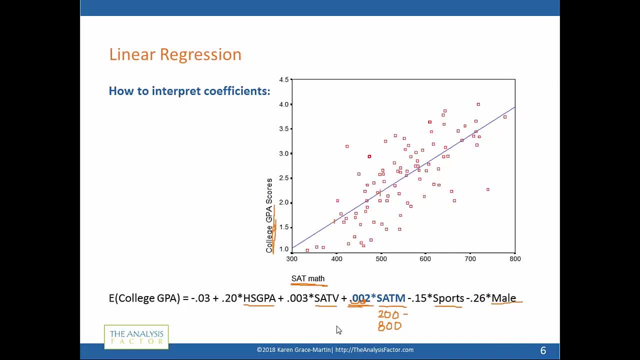 well for a 100 point increase in SAT math. on average we see a 0.2 increase in GPA and that's actually a noticeable difference in GPA, right? So that would take somebody from a 2.5 to a 2.7.. 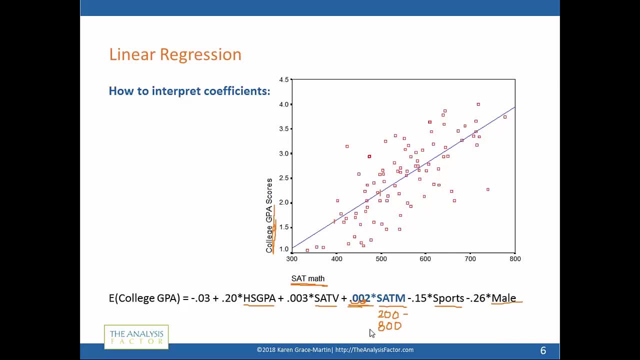 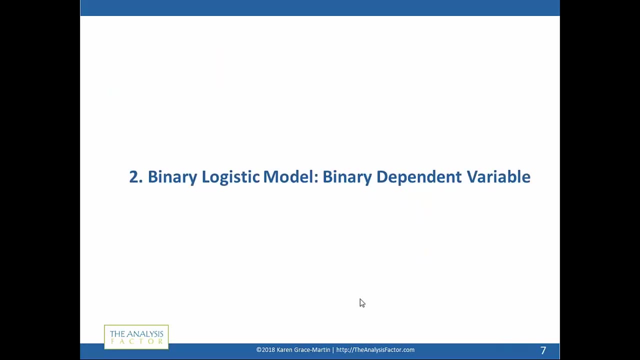 That's a noticeable increase in GPA. So SAT math is actually a very significant increase in GPA and it's actually predicting GPA. although it doesn't, it looks like it has a very small coefficient. Okay, Let's talk about a binary logistic regression model. 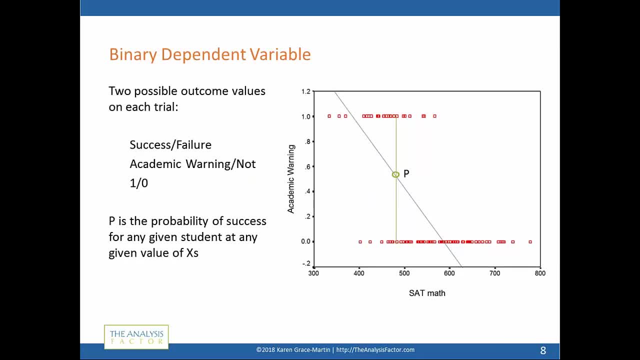 Okay, so the key difference here is the dependent variable. Okay, instead of having a score for each individual, we have a binary categorical variable. Okay, so that means we tend to think of binomial distributions as a set of trials, And in this situation, each student is a trial right. 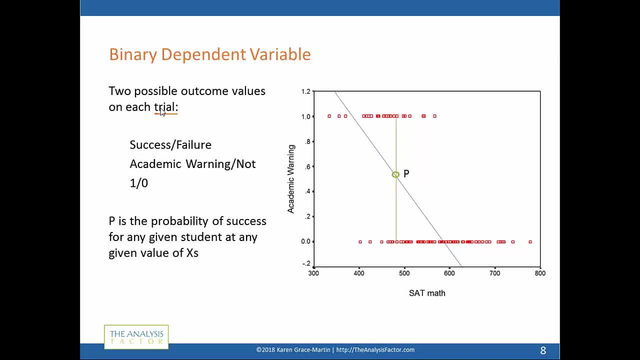 And that the outcome of each trial is either a success or a failure. Okay, so we're not focusing on GPA and again, maybe as the admissions counselor, or maybe you're not in admissions, maybe you are in the tutoring center or something. 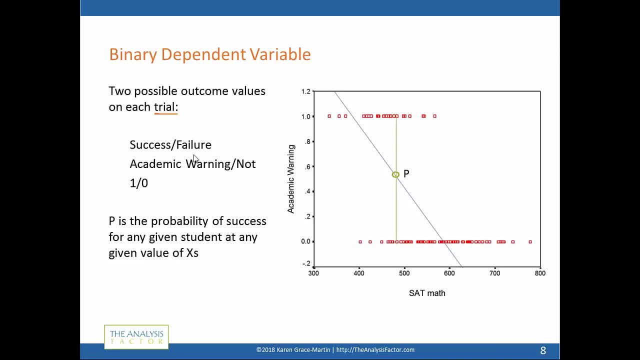 and you are trying to identify who are the students who are in trouble for going on academic warning, maybe after the end of their freshman year, So the students who are going to struggle. So we're not really interested in their specific GPA, we're interested in 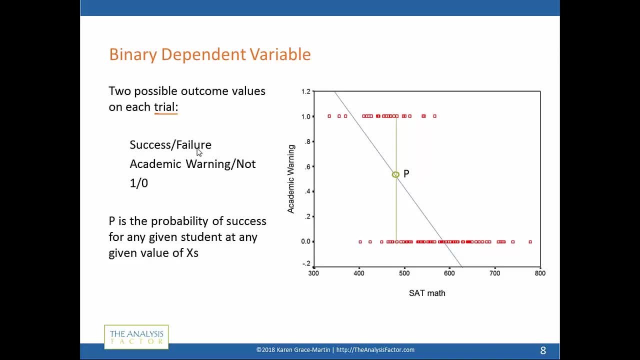 are they going to have trouble? Okay, Are they going to pass their classes? So we only have two outcomes: success and failure. Now, in logistic regression terms, success is usually defined not as the better outcome, but the outcome category that we're more interested in finding or in predicting. okay, 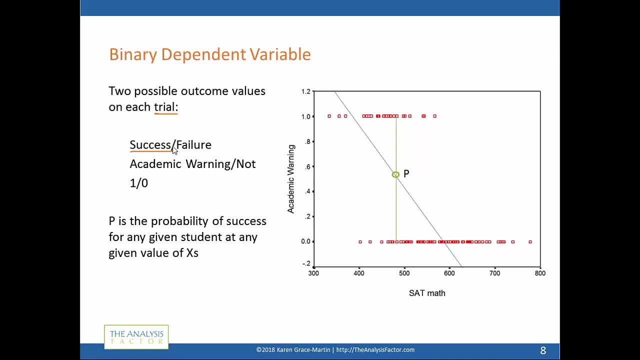 Now it's a little bit like two sides of the same coin, right, Because if somebody doesn't go on academic warning, they're just the other side of a success. But here we would want to talk about it in terms of what predicts the probability. 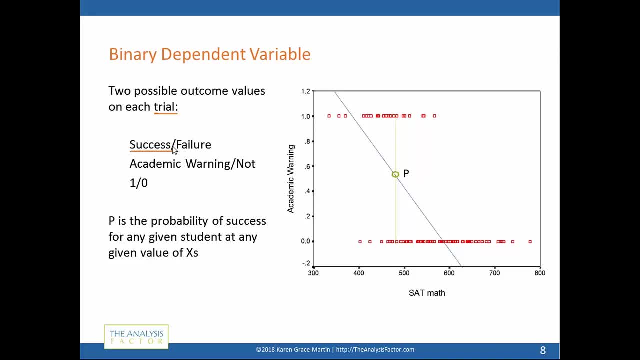 of going on. academic warning. So academic warning, even though it's the worse outcome in terms of you know how the students feel about it. that's what we're going to call a success. Now you will notice, we give these two categories, you know. 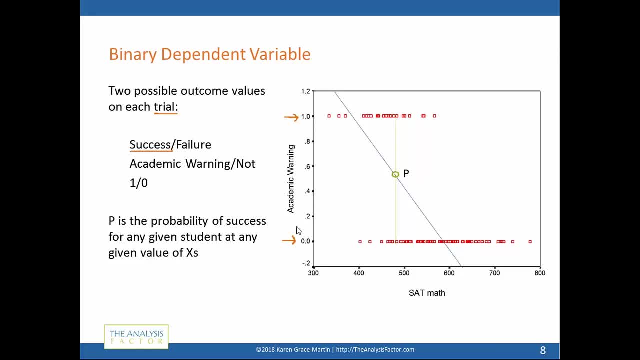 categories, numbers, numerical values, and it's just coding, And they're coded as 0 and 1 for mathematical convenience. When we do it this way, it makes the equations work out nicely. That's really why we use 0 and 1.. 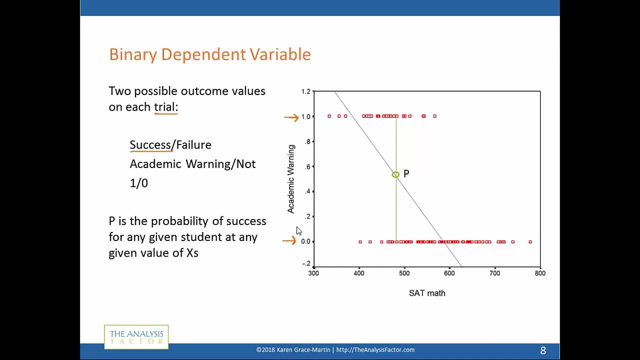 But they really are arbitrary and essentially we're not truly interested in predicting if any given student goes on academic warning or not. But what we're interested in is the probability that a student with a given SAT, math, SAT, verbal, high school GPA, how we can use these predictors to predict the probability that. 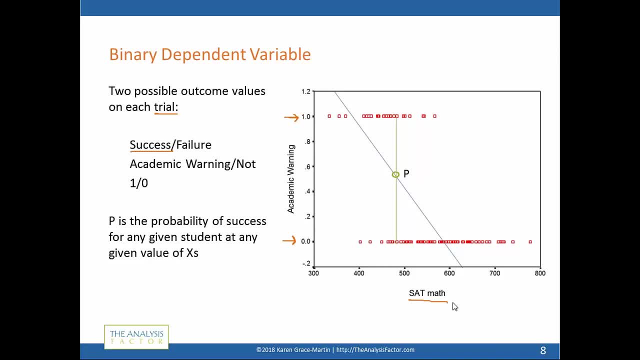 any given student will go on academic warning 0. And you can see from this blue line here, if you try to fit a line, just a linear model, it doesn't work. It is not at all telling you anything about the actual values of academic warning, or even. 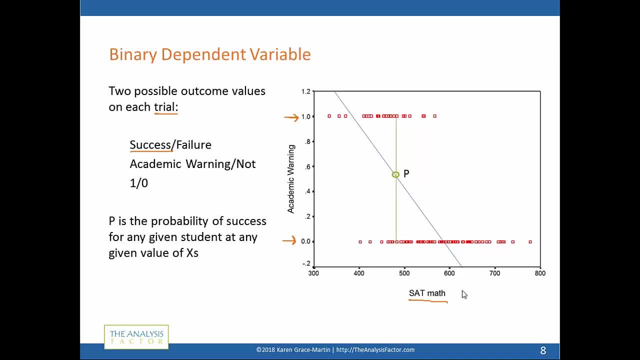 very much about the probability for any given student. If we actually were to plot the probabilities for any given student, it would look like this: Right, Because you can see, we generally estimate probabilities from the proportion of the data. So pretty much everybody who got maybe, say, 600 and above, they did not go on academic. 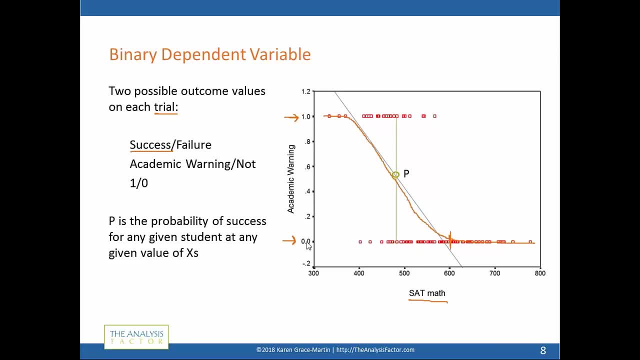 warning, They ended up with an outcome of not academic warning. They're down here And everybody at the very lowest SAT math scores ended up on academic warning. But then we have this group here in the middle right with a probability of going on academic. 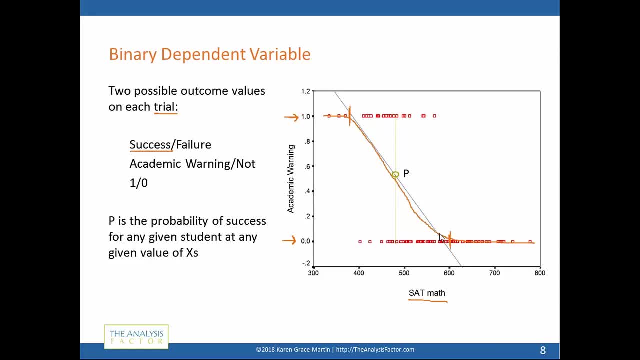 warning That's neither 1 nor 0. Okay, It's something in between, And technically these are not quite touching 1 and 0. They're really asymptotes, but they're getting very close to 1 and 0.. 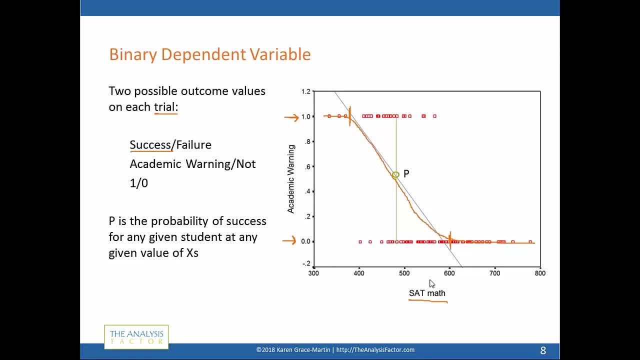 But in between, So we can use. we can see that there's still a relationship here. Right, The higher the value is, the lower the overall probability. Okay, And we get this probability really from the proportion of students at any given math score. 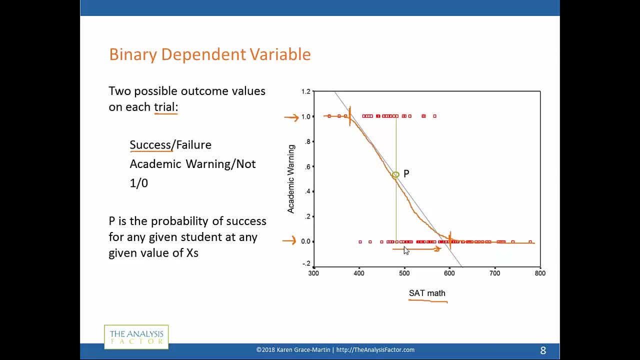 SAT math score. Okay, I'm going to pause for just a couple minutes And answer some questions. Yes, the 01 binary variable is nominal. Yep, I mean really with only two categories. when it's categorical, you can't have ordering. 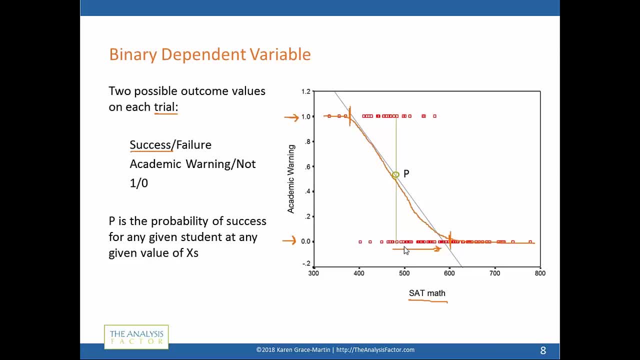 really Ah. So Jerry asks: why is the green line in the green point Draw on where it is? I'm just saying it here. If you take any given value of x, there's a point in between Right, The that gives you the probability. 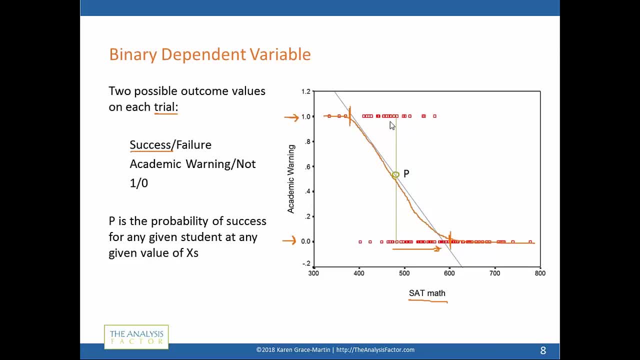 Because any given student, even if they have, say, a 0.52 probability, some of them will go on academic warning and some of them won't. So you can't calculate this probability. You can't calculate this probability with just one per student. 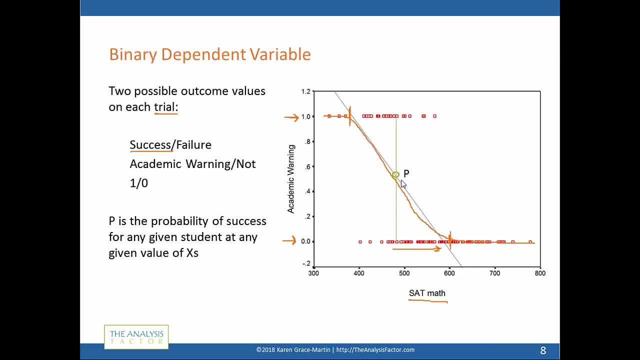 It's really a group, a grouping variable, And really it's. it's the mean. It's the mean of the 0s and 1s. Okay, And, as I mentioned, logistic regression is a type of general, generalized linear models. 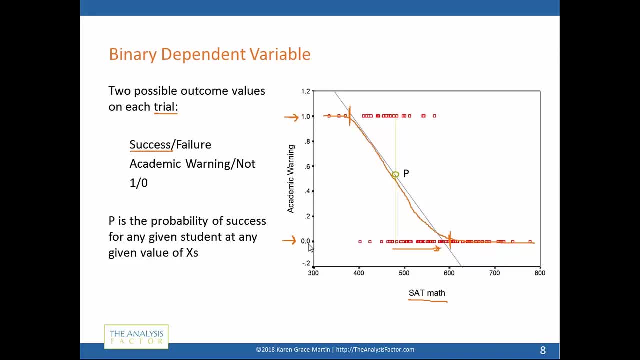 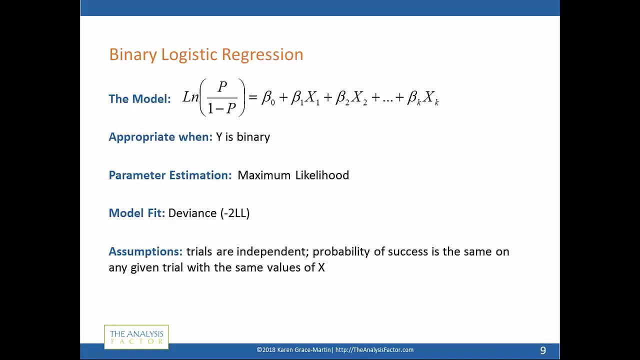 And all of them have one. All of them have what's called a link function, which is a function of the mean of y. So we are not directly modeling the values of y, but a function of the mean of y. Okay, That function looks like this: 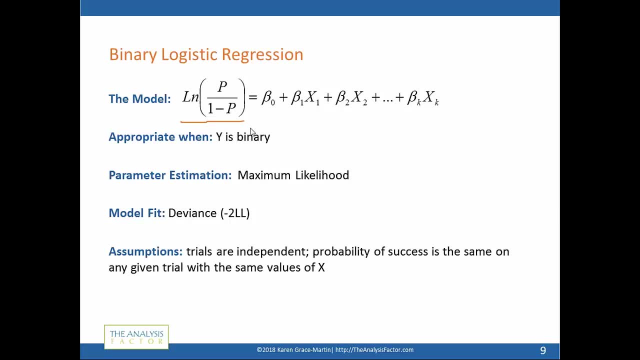 And if you're not used to that, that looks a bit ugly, Although the right side looks beautiful Right. So the right side of our equation looks exactly like our second linear regression model. Right, Nice linear form. We have the intercept. 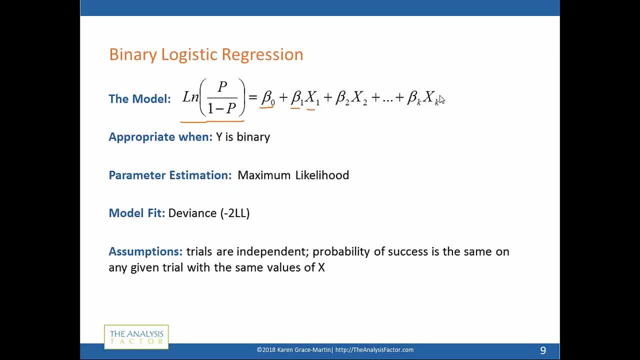 We have beta 1, x1s and so on, So that side is all good. The only thing that's really changed in the model is we've taken this function. it's called the logit function and it's the log of the odds of success. 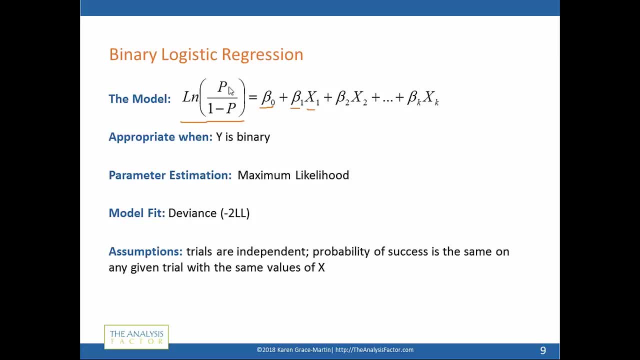 Now the odds is calculated from the probability. Okay, So this p is a probability of success for any given student on any given trial, And when we put p- probability of success- over the probability of failure, which is 1 minus p, we get the odds. 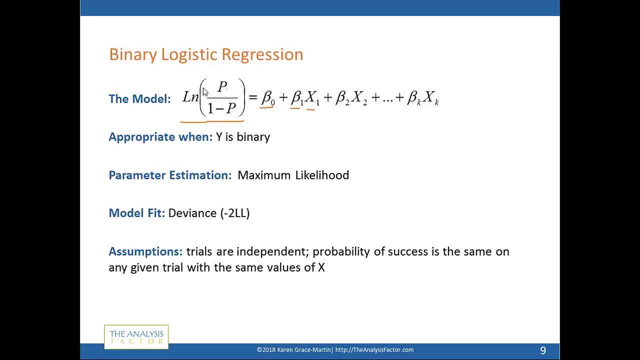 And we'll talk a little bit more about odds. But suffice it for now to say that the probability of failure is 1 minus p. But suffice it for now to say that the log odds is a function of p Right, It's a function of the mean of those 1s and 0s. 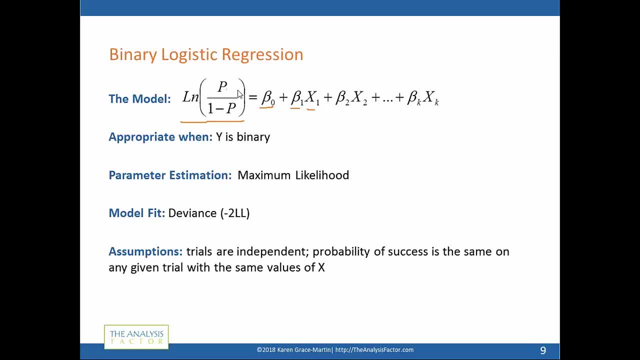 And we have to use this function, this link function, in order to set up the model in this nice linear form. And we set up the model in this nice linear form so that we can do the calculations necessary to estimate our parameters. Now, once we get those estimates, we can back, transform, if you will, our regression coefficients. 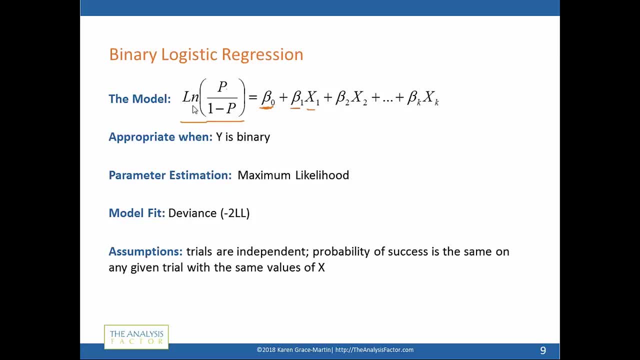 in order to make them make a little more sense, Because most of us can't think on a log odds scale. So this is the model. Let me explain this And then, on our just a moment, we'll dig into odds a little bit more. 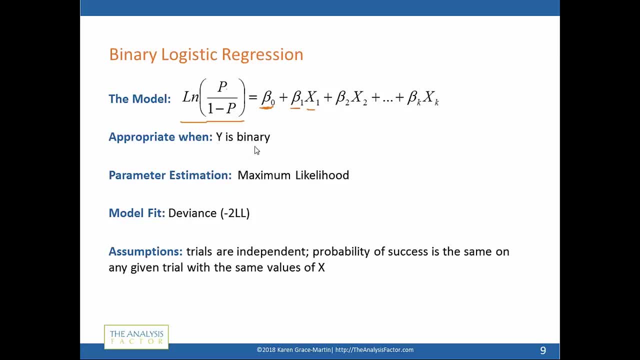 Okay, So we use it. when y is binary, Two outcomes- success or failure- For any given person, there are only two outcomes. They are mutually exclusive. Okay, Nobody can be in both. have both outcomes. They must be mutually exclusive. 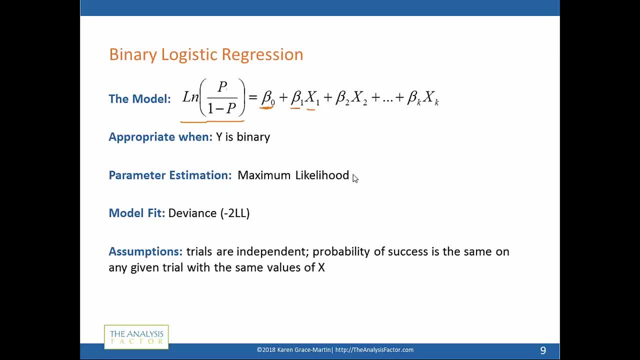 Here. this is key. This is really important in many ways And you will have seen this before if you've ever used structural equation modeling or mixed models Instead of least squares estimation. because we have a more complicated model, we can't use least squares. 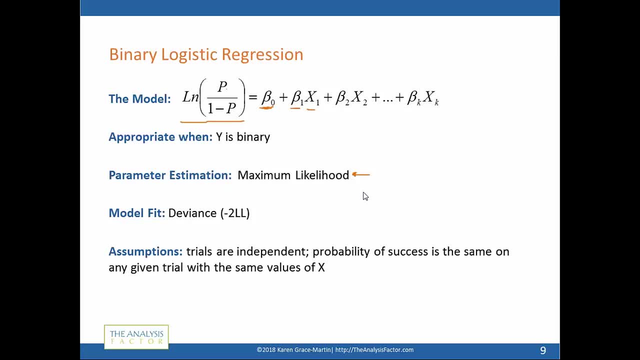 Least squares is an algebraic solution. Okay, You can actually, if you really had nothing else to do on a Saturday, could sit down and calculate least squares estimates using pencil and paper. You cannot do that with maximum likelihood. It's an iterative process. 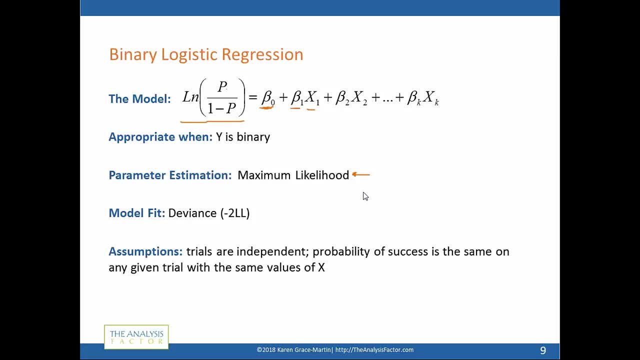 It's an iterative algorithm and it uses calculus. It's much more complicated, but it has all the same properties as least squares, And it turns out that if you end up in one of those simple situations, like a linear regression, where you could use least squares, you will get the identical results from maximum likelihood. 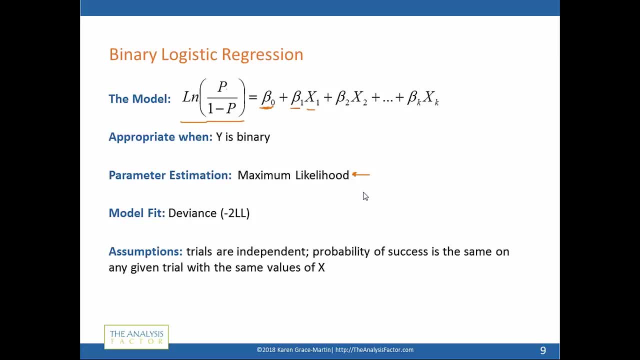 as you do from least squares, So this is actually considered a subset of maximum likelihood. The biggest disadvantage of maximum likelihood is that we can no longer use R-squared to measure our model fit. There are many of alternative statistics, including this deviant statistic which is: 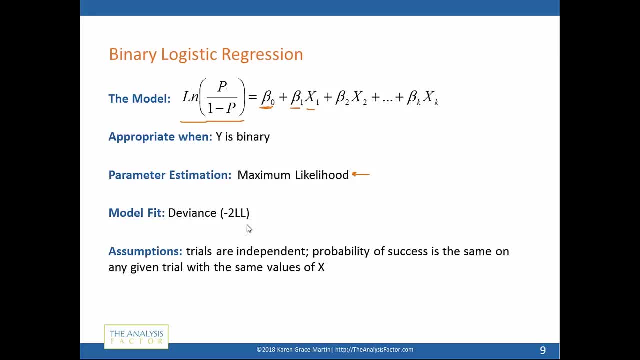 probably the closest equivalent to R-squared, But there are others. There are others like AIC and BIC, other information criteria. So there are ways to measure model fit. They just are not. they don't have the nice intuitive interpretation that R-squared has. 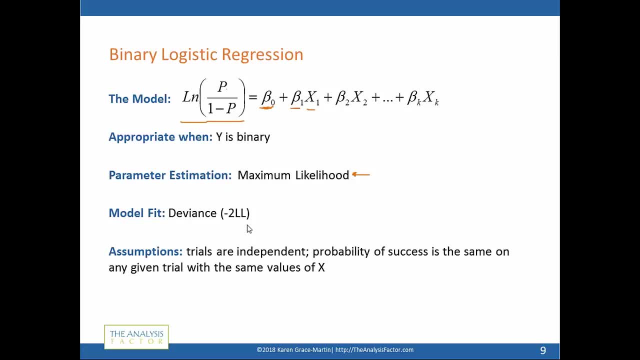 Okay, So the big assumptions here in binary logistic regression is that our trials are independent of each other, So the fact that one student goes on academic warning is not affecting others. Okay, Their probability of going on academic warning In a data set like this, if they're all at the same college, that might not be the best assumption. 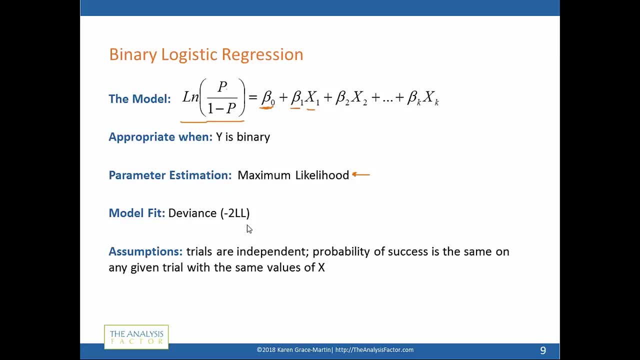 and we'd have to dig into it a little bit. However, let's just assume we've got it here That it is something you should consider. But the other big assumption is that the probability of success is the same on any given trial, given X. 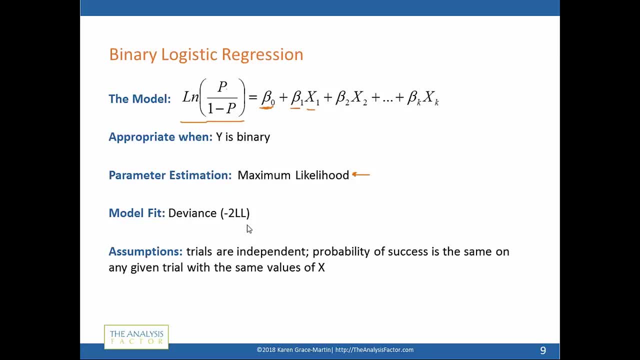 Okay. So if we have two students with the exact same high school GPA, the exact same SAT math score- both are male and neither did sports- we would expect the exact same probability of going on academic warning. There's not something else going on above and beyond. 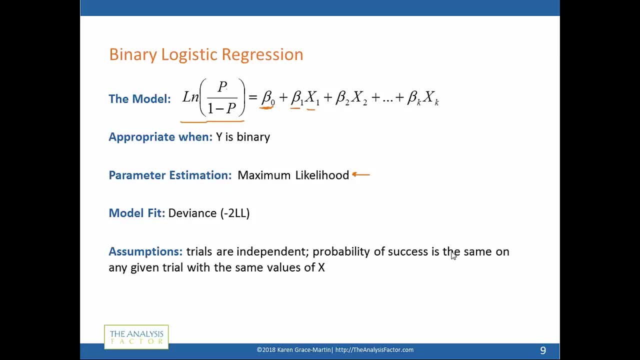 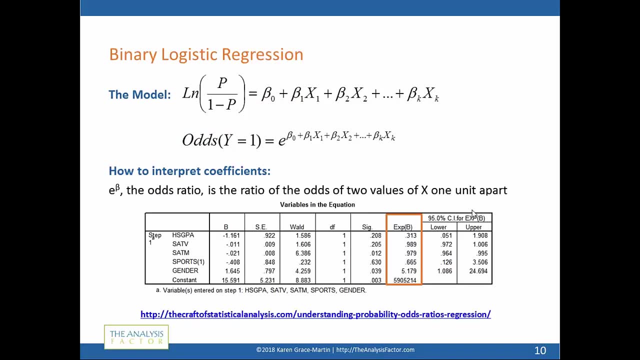 It's yeah, Okay. So let's see the model a little bit in action and let's talk a little bit more about odds and odds ratios, which are a key concept in logistic regression. I will, before we even start, I'm going to point out this link at the bottom: 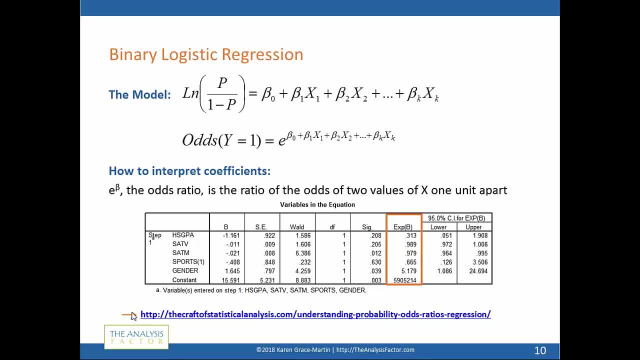 This is another free webinar we did in this Craft of Statistical Analysis series where it's entirely the whole thing is just on probability, odds and odds ratios. So I recommend you take a look at that if you want to dig into this even more. 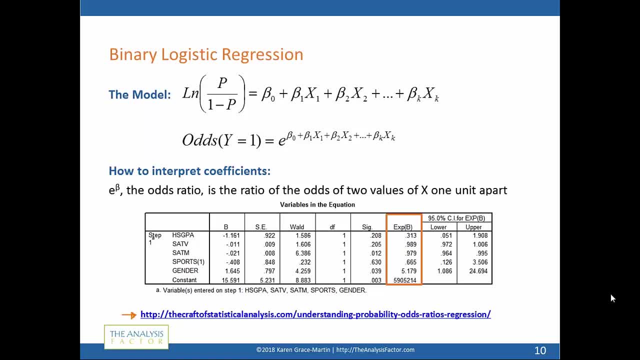 because we can really only do a quick overview here And there. we spend, you know, a whole hour on it. But here, as I said, we've got this logit link function over here on the left. Okay, And it's the log of the odds. 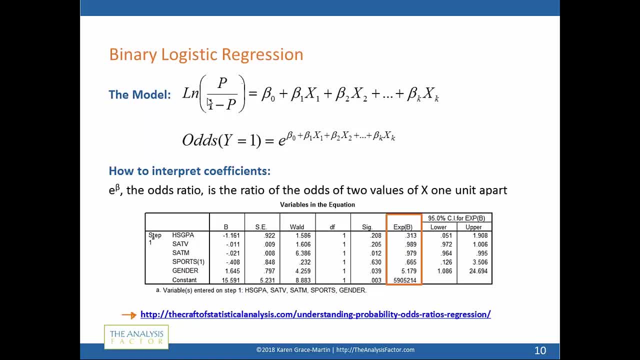 So this whole piece right here, this p over 1 minus p, that's called the odds. Now, odds are a tricky thing because in conversational English people use the terms probability and odds interchangeably. They are not the same thing mathematically. 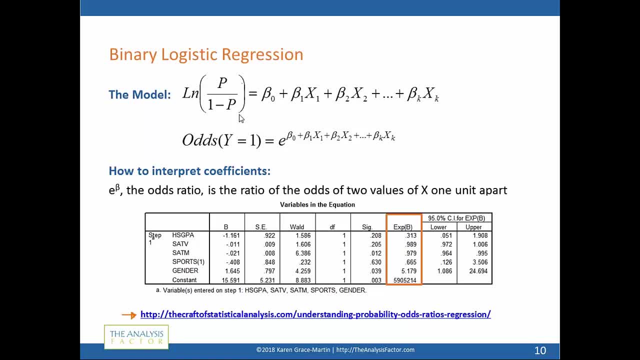 They are both measuring the same thing, But they're not actually on the same scale. Okay, So probability is something we're all more familiar with. It ranges from 0 to 1.. It's the number of successes out of the total number of trials. 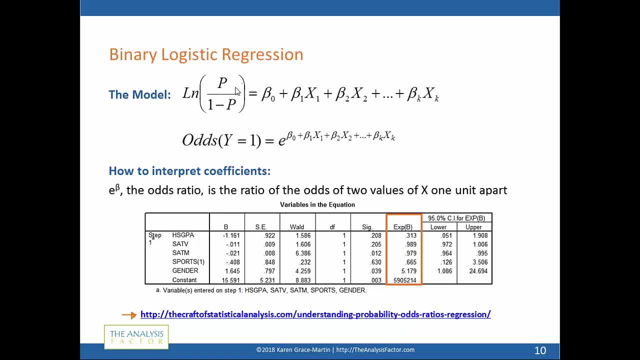 Odds range from 0 to infinity, And they are the number of successes divided by the number of failures. Okay, It turns out that's equivalent to this with p over 1 minus p. Okay, So it's the probability of success divided by the probability of failure. 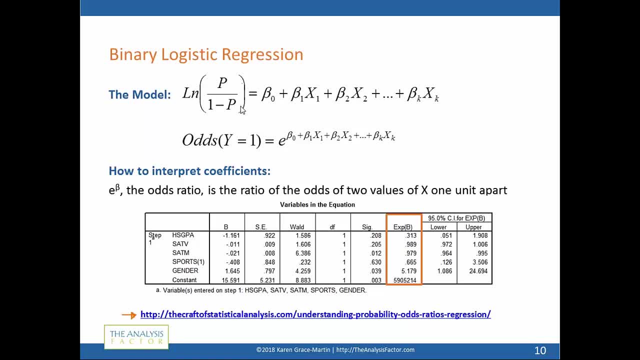 Okay, The only thing I've ever seen people really truly use odds for for the most part is gambling Right, You hear about odds of winning the lottery or odds of a horse coming in first. I'm not sure why we use odds there, but virtually everything else in life you hear about probabilities. 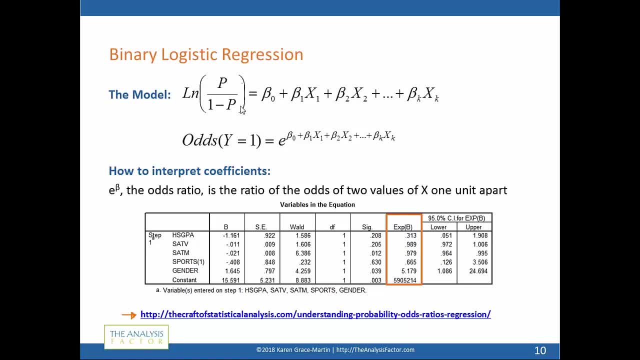 So it's one of those things you want to be aware of. You don't want to interpret an odds as if it were a probability, just as you don't want to interpret 30 degrees Celsius as if it were 30 degrees Fahrenheit. Okay, 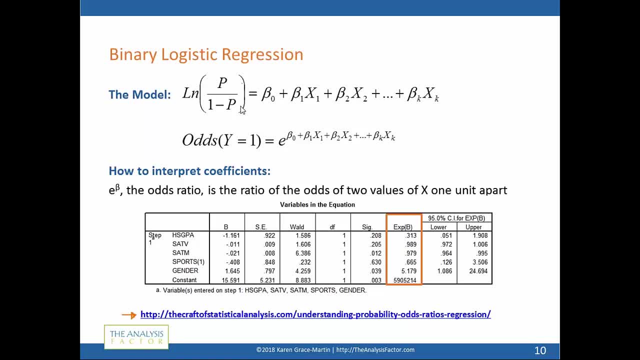 They're both measuring temperature, but on vastly different scales. Same thing here: They're both measuring how likely a success is, but on different scales. Okay, And as I said in this other webinar, we go into it a lot more In my logistic regression workshop. we go into it a lot more because really understanding odds is important. 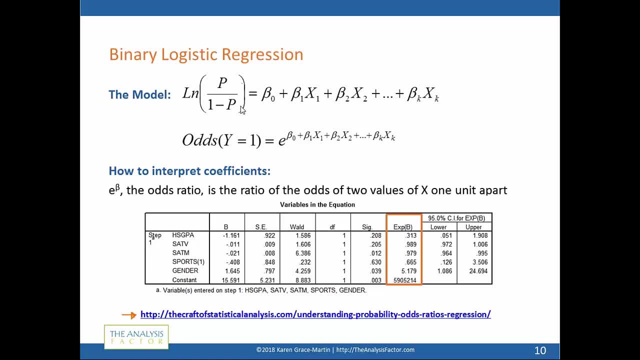 A lot of people say it's too hard and they can't learn it. I disagree. I think everyone can learn it. It just takes a little while because we're not used to it. So what makes it even harder than that is: not only are we dealing with odds, 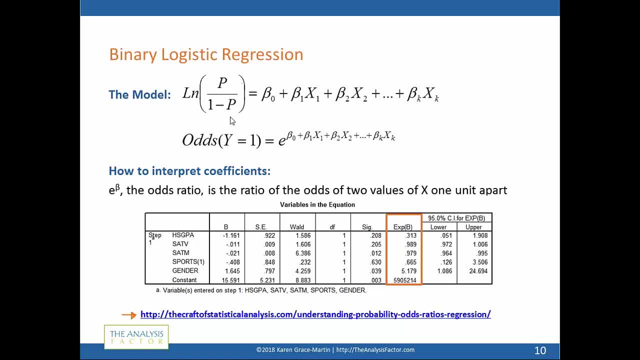 but we have to take the log, the natural log of the odds, which you know. now we've added another whole complication. Okay, Because logs are hard. It's hard to think on a log scale And for many of us, 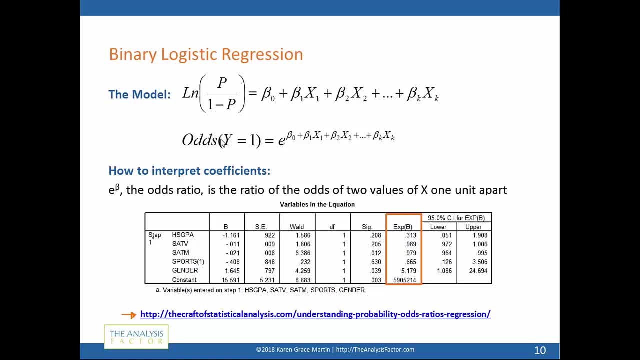 it's been a few years since we covered logs in. you know high school algebra, So if it's not, you know, fresh in your mind, it can make it seem completely overwhelming. That said, if we break it all down, it's not so bad. 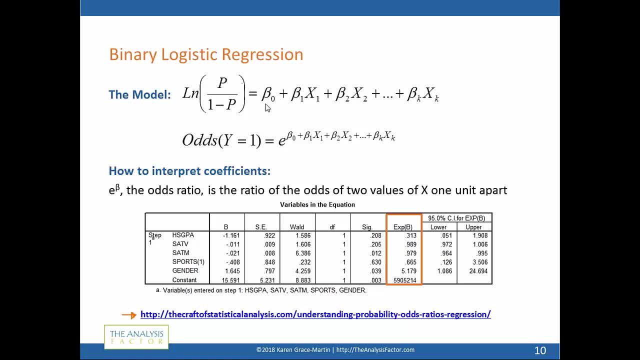 So, once again, we estimate the parameters with the model in this form, but it's not how we're going to interpret them. We're going to interpret them in this form. This second one: here You can do the algebra if you want to. 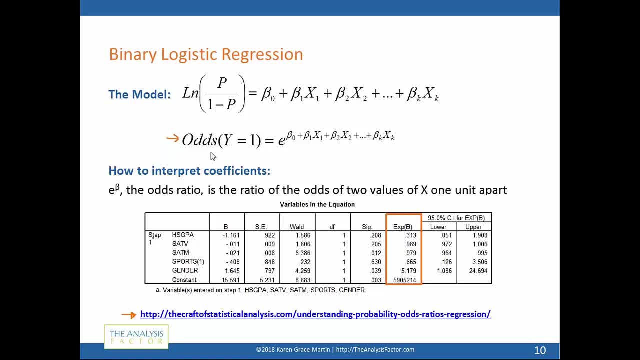 and you'll see these are equivalent And essentially it's saying the odds, that y equals 1, the probability over 1, minus the probability equals this stuff over here. Okay. So first of all, what the heck is e? Okay. 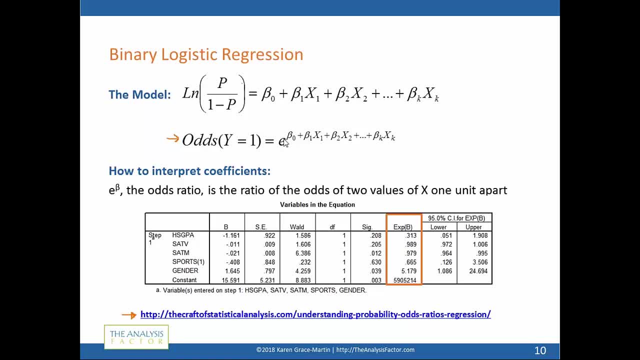 E is a constant, So, just like pi is a constant, e never changes. It is the inverse function of a natural log. In fact, we just did a webinar again, a 90-minute webinar- on what logs are? We talked a lot about e. 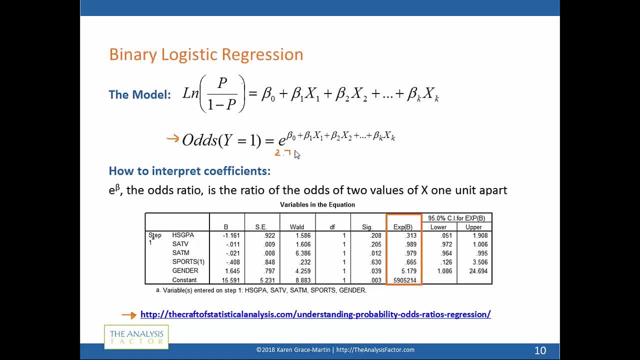 E is approximately 2.72.. But essentially what's important here is e raising something. e to some power is also known as exponentiating that value. So here we have raised e to the power of my entire right side of the equation. 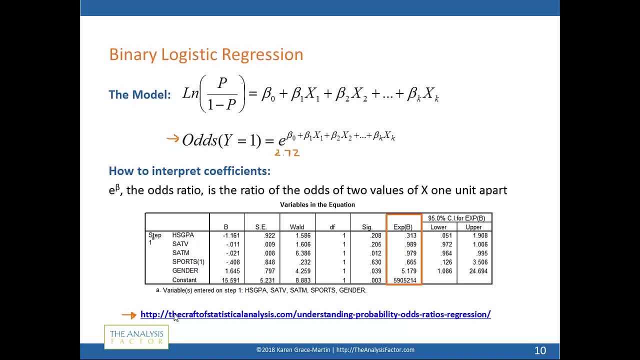 And what that does is it gets rid of the log. Essentially, what I'm doing is I'm raising both sides of my equation to e right And these cancel out because they're inverse functions of each other. So I end up with just odds and I end up with this messy thing over here. 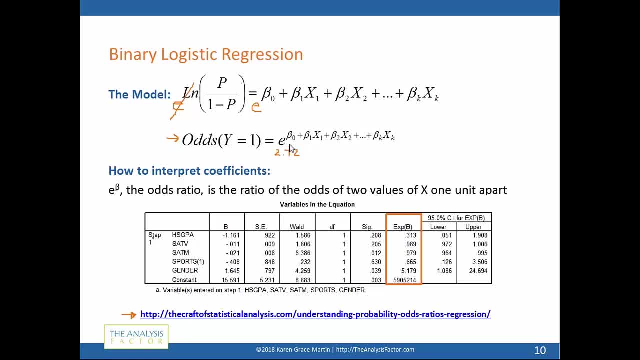 Okay, Well, luckily the way the algebra works, when we exponentiate something, we can exponentiate each one of these betas on their own and get these values in this column right here. So my software did it for me. So over here I have b's all the estimates of each parameter. 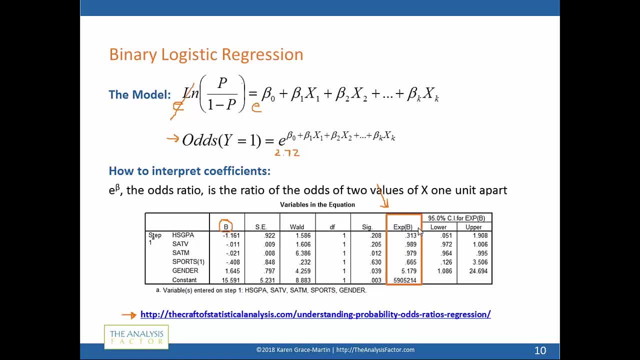 And here I have the exponentiated version of those. And let's once again focus on SAT math. So we can see here, if we wanted to try to interpret this, that would say, for each one unit increase in SAT math, the log of the odds of going on academic warning goes down. 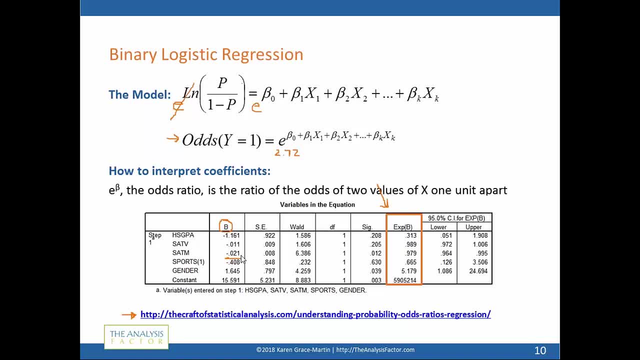 It's negative, so it goes down by 0.021.. Okay, And that is a linear function. We actually have a linear function between the log odds and everything over here on the right, So that's a linear relationship. But the problem is: virtually nobody can think on a log scale. 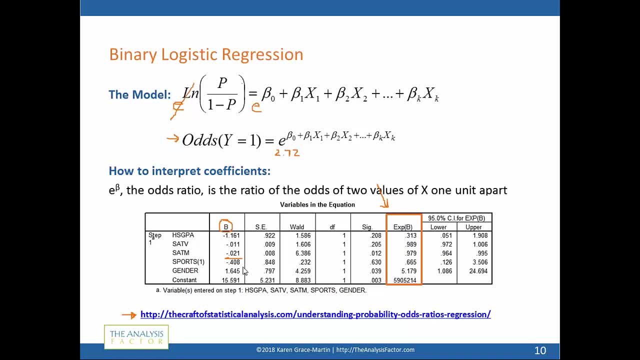 So that's not meaningful at all. besides the fact that it's negative, It's a negative relationship. As SAT math goes up, the log odds of going on academic warning is going down, So people are less likely to go on academic warning. 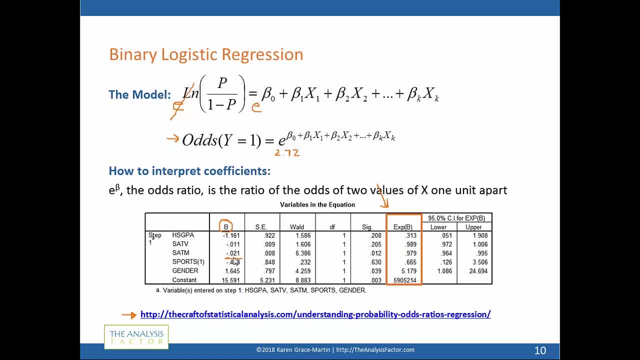 But the actual size of it it's hard to interpret. So we exponentiate, So we exponentiate it, And when we exponentiate it we're getting rid of the log. Okay, So we've gotten rid of that log. But again, remember here, what we're doing is we're saying: 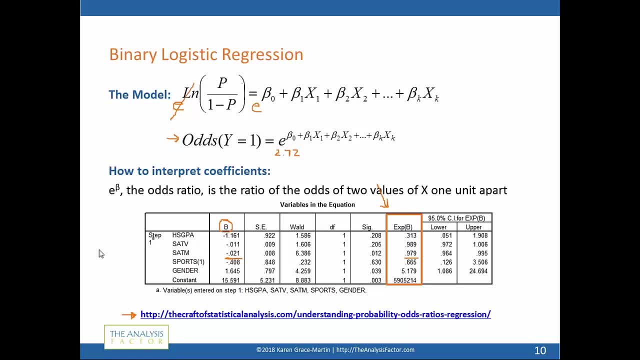 okay, how much does y differ? You know change in y over change in x, Right? So when x changes by one unit, so a one unit change in x, y changes by negative 0.021.. That's a difference, right, between two different values of the mean of y. 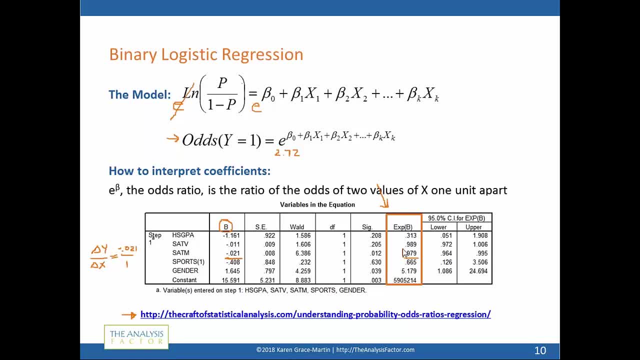 Well, here once we. because we're getting rid of the log and because logs are, at their heart, exponents, they mess up the algebra. So instead of having a difference in y, we have a ratio, So x is still changing by one unit. 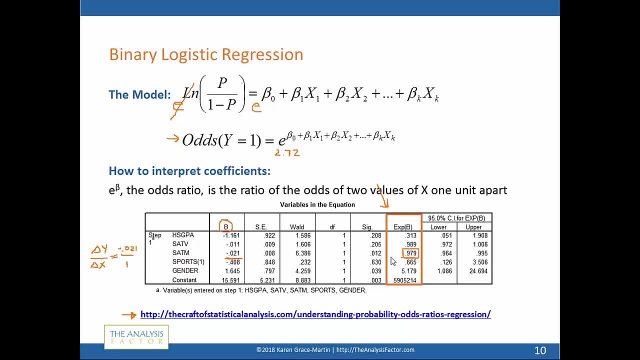 But y is a ratio. So what this says is for every one unit increase in SAT math score, the odds that a student goes on academic warning gets smaller by a ratio of 0.98.. So, for example, if we have two students whose math SAT scores are one unit apart, 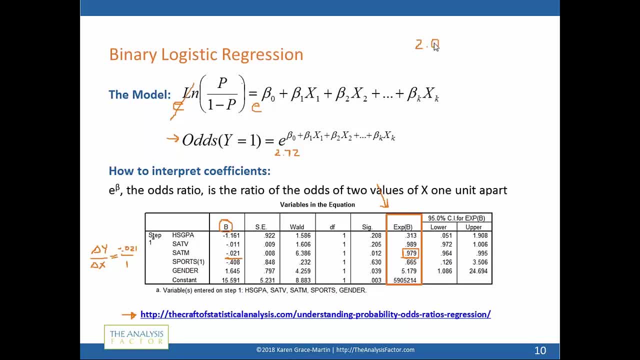 and one of them has a GPA. or let's say, on average, the GPA is 2.0.. Sorry, not GPA. Let's say the odds of going on academic warning is 2.0.. And then my next student, whose SAT math score is one unit higher. 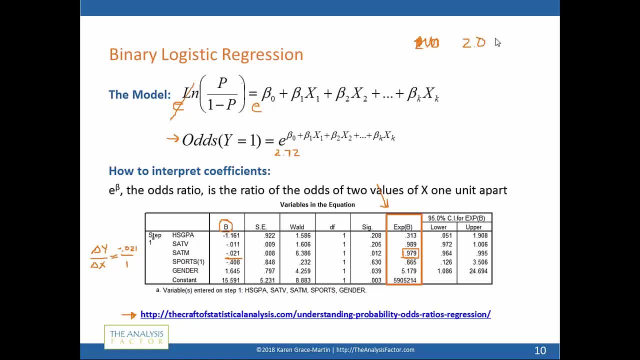 well, their odds will be 2.0 times 0.98, which is going to be slightly smaller, right, It'll be what? 1.96?? So slightly smaller. So, as the SAT math goes up, the odds of going on academic warning is getting smaller and smaller. 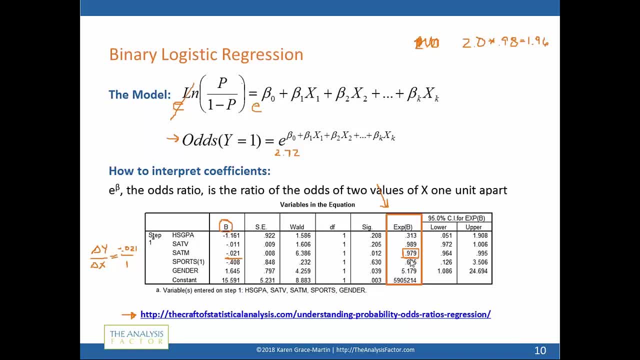 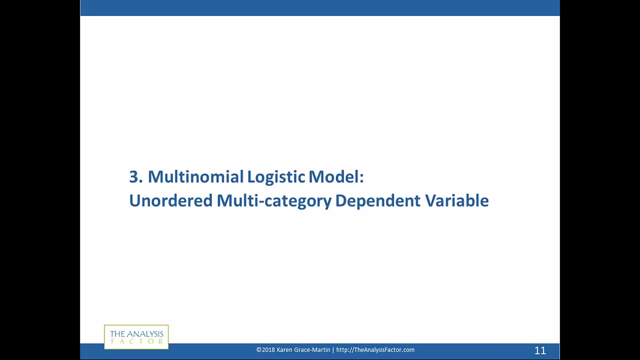 by this factor of 0.98.. Okay, So it's a relative change. It's really a ratio or a rate change is how you can think of it. So it's not a change by addition, It's by multiplication, And again we have lots more resources on really digging into what an odds ratio means. 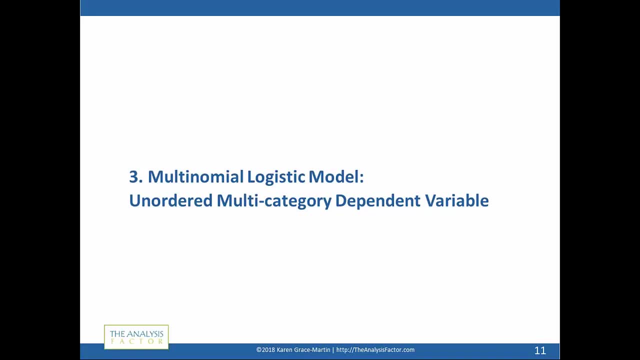 And so I recommend you take a look at those. Let's pause. Yeah, we should have time. I'm going to ask a couple questions. Okay, Yeah, Samrat says odds of going on academic warning goes down by approximately 3%. 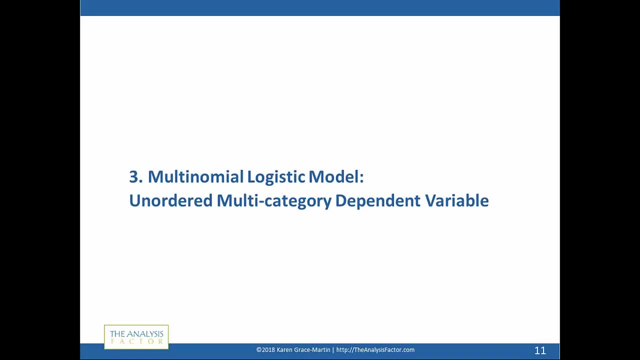 with a one unit increase in SAT math. Is that a correct interpretation? It is, Ah great. Brad asks how odds ratios can be used as effect sizes. How would we interpret the odds ratios in your example in that light? That's really exactly what we were doing. 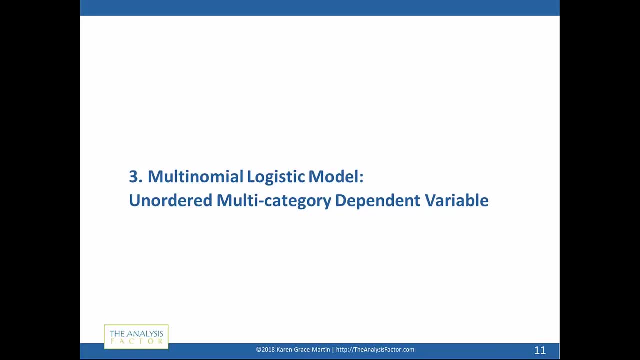 was trying to understand: how big is that effect? Okay, So that's why it's so important to understand what an odds ratio really means. Now, it is an effect size, but it's not necessarily a standardized effect size, which is what people often want. 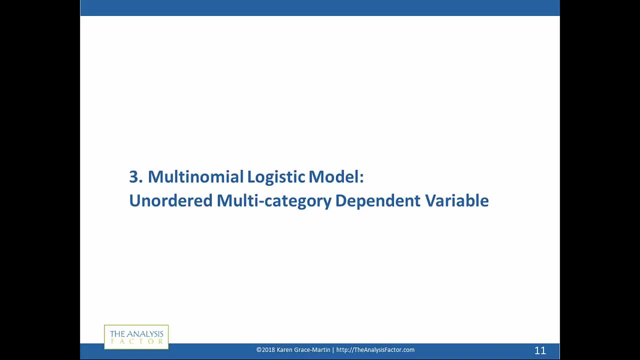 so it's not equivalent necessarily to a correlation or a Cohen's d, unless we standardize the x variable. So here we were talking about a one unit change in x. If we wanted that to be a standardized effect size, we'd have to basically turn our SAT math into z scores first. 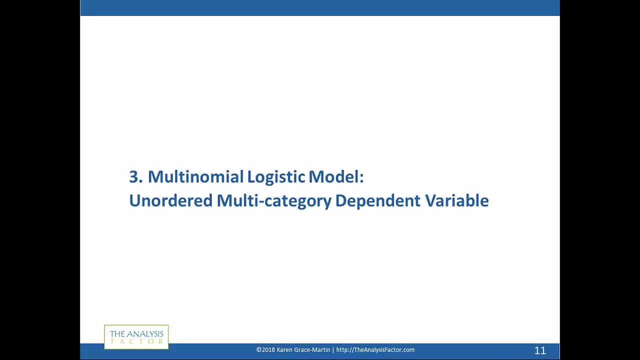 We'd have to standardize those. Okay, There are more questions and I will come back to them at the end, but I want to make sure we get through everything. So let's talk about multinomial logistic regression. So now we still have a categorical dependent variable. 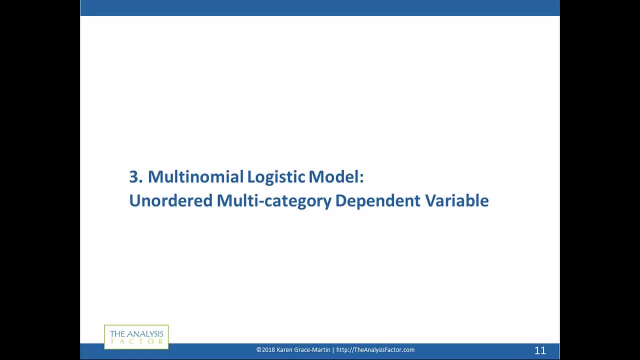 but there are more than two categories- Okay, three or more. So in many ways it's exactly the same. We're going to set up the model in a very similar way, but we have more categories to work with, So it gets a little bit more complicated. 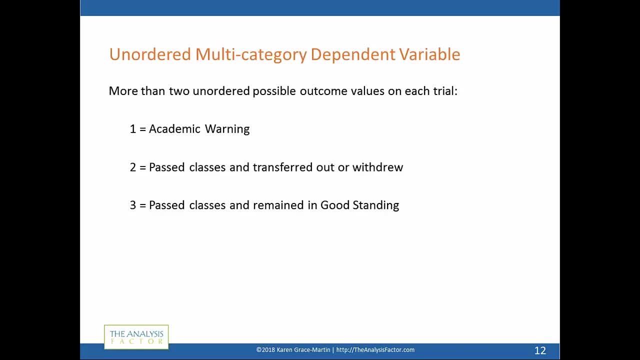 Okay. So here's an example of again. maybe there are more than two outcomes, Okay, Maybe one of them is still going on academic warning, And a second outcome that maybe the college cares about is that, yes, they passed all their classes. 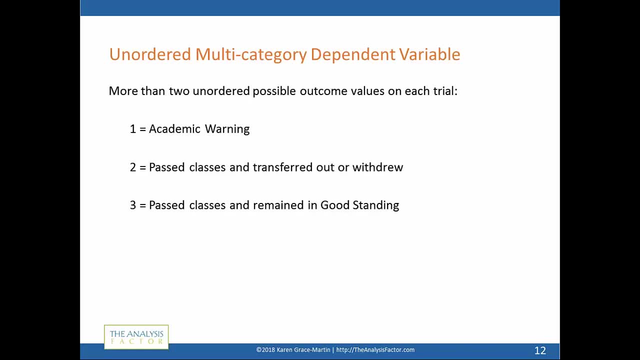 but they transferred to another college or they dropped out, So they're not. it's not the same as passing all their classes and staying, So there are different outcomes for their students. Ideally, as far as the college is concerned, they want everyone in category three here, right? 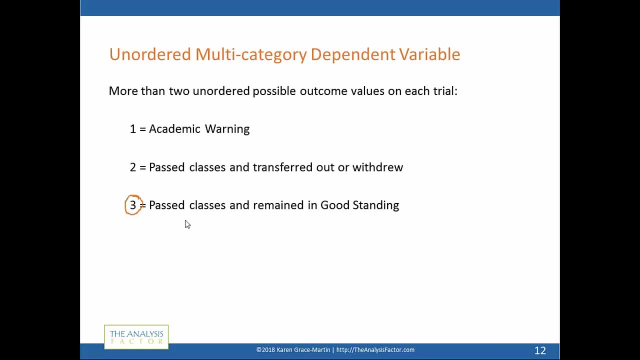 Passed all their classes and they stay at the school and they're in good standing. But there's not really an order to the other two. These two are not. you could say that one is worse than two, but maybe not, You know, maybe from the college's point of view. 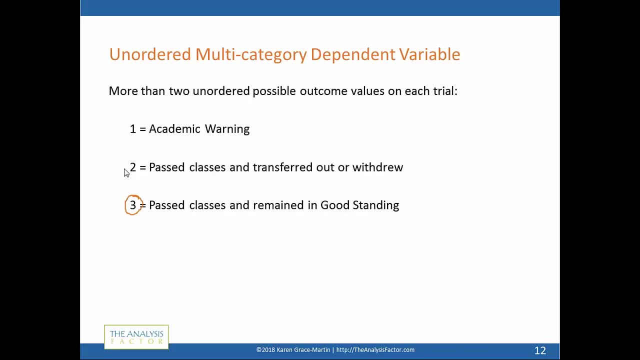 they really view them as just three different outcomes And if you do want to assume an order, you have to be very clear that they really are ordered, And I don't think I could make that assumption here. So there are really three nominal categories, unordered. 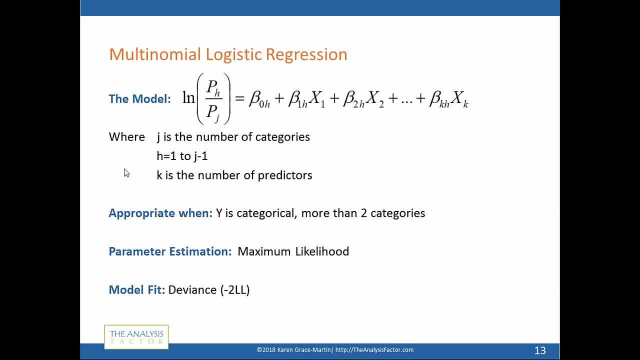 Okay, So you will notice. the right-hand side of the graph equation looks almost exactly the same. There's only one difference And we have an extra subscript over here: H And H is the number of categories. Okay, But the other thing. 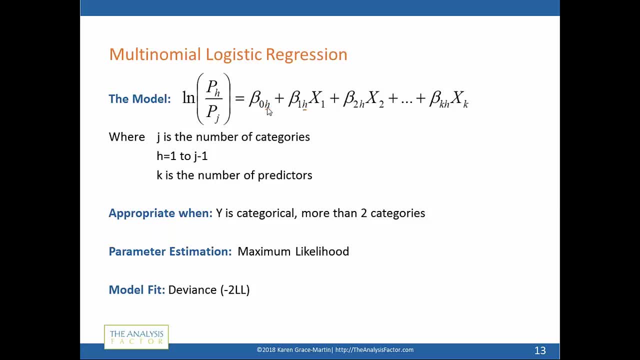 oh, I'm sorry. H represents each categories, starting at one and going up to J, where J is the number of categories. sorry, So our J is three here. right, We have three categories, So H can have values of one or two. 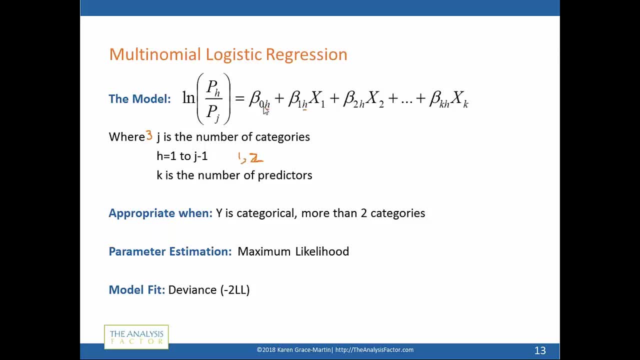 Okay, So we have two. what that indicates here already, as you can see, that means we have two sets of intercepts: beta naught one and beta naught two. We have two effects of H1. And it's because? what multinomial logistics. 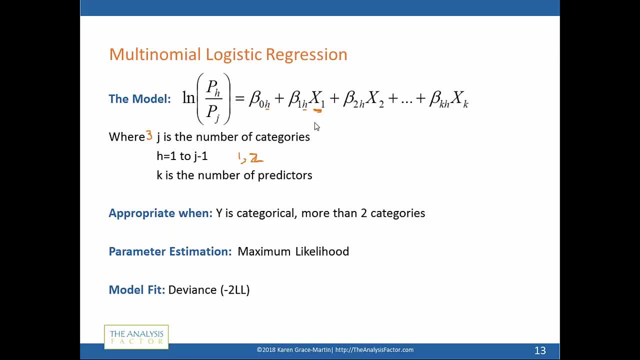 regression is doing is literally simultaneously running two binary logistic regressions on our three categories, And they're always comparing the probability of one of the categories to the last category. Now, last is totally arbitrary, It's whichever one you assign to be last. 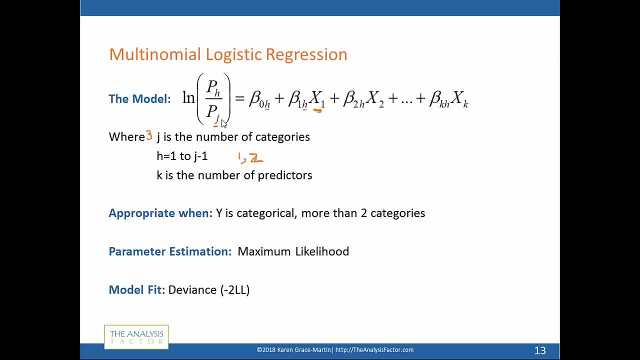 which makes the most sense. In our case it was being in good standing and remaining at the college. So this is P3. So when we set up the odds, it's not the probability of academic warning compared to not academic warning, It's probability of being in. 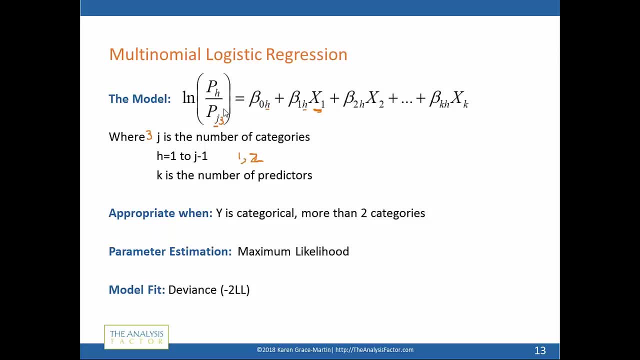 going on academic warning compared to the probability of remaining at the college in good standing. It's a very subtle difference, But if we did the first one, actually the model would not be identified. We would not be able to calculate anything. We'd have no estimates. 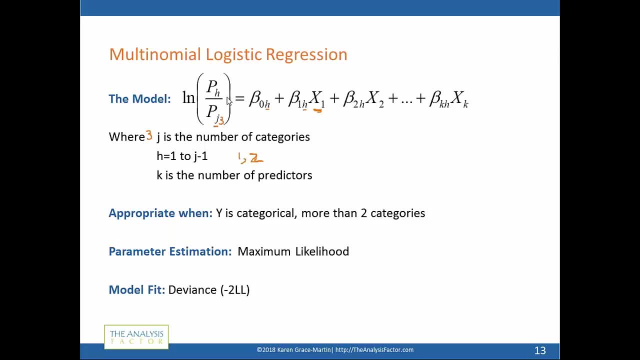 Things would be confounded, So we have to set it up this way. But essentially, and when you ever look at output, you just have to interpret everything in terms of category one compared to category three. What's the odds of being in this category? 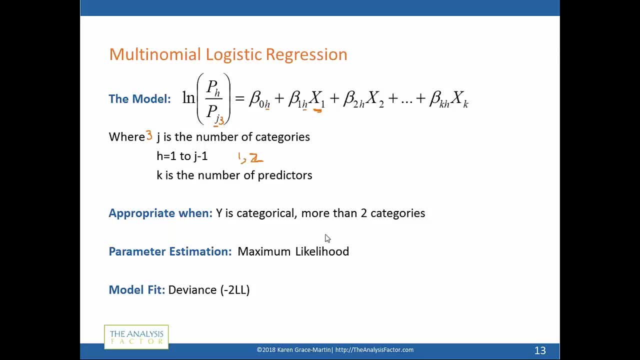 versus that category. It's still a log of this odds Again, we already talked about this- When we have more than two categories, the other stuff stays the same. We're still using maximum likelihood and we are still using deviance to measure model fit. 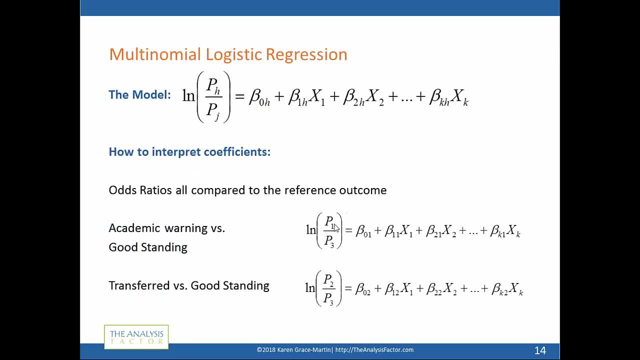 Let's look a little bit closer, So here you can really see what's going on with it. So we have two full models. One is looking at the probability of being on academic warning compared to being on good standing, And the second one is: 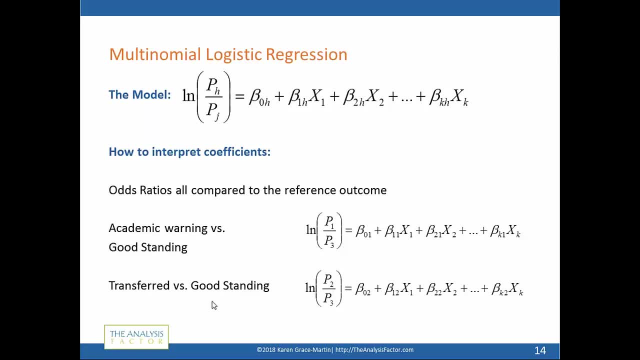 what's the probability of transferring versus remaining on good standing? The effect of the predictors might be different. You will notice the entire set of coefficients, the intercepts and the effect of SAT math. Maybe SAT math has a big effect on whether someone goes on academic warning. 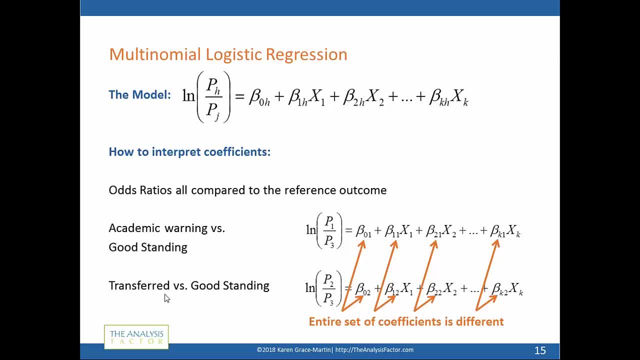 versus good standing, but has no effect on whether somebody transfers or stays on good standing, So we can have completely different effects. So the advantage of that is we have a lot of flexibility in these models. We don't have to make many assumptions. 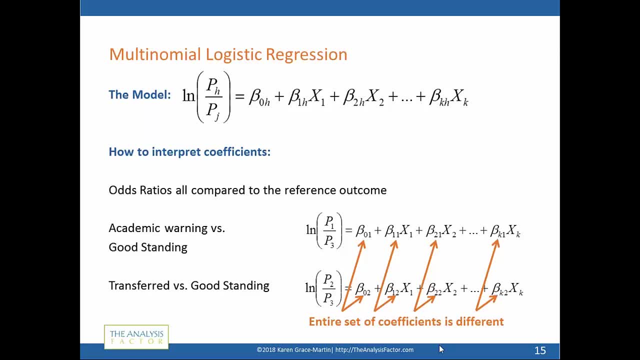 The disadvantage is, if you have a lot of outcome categories, you're going to get a lot of output, And sometimes when there's a lot of output, it's a bit intimidating and it's hard to see what the patterns really are. So it's good in that we have 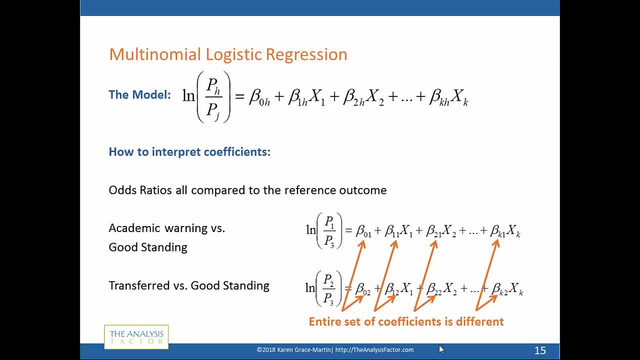 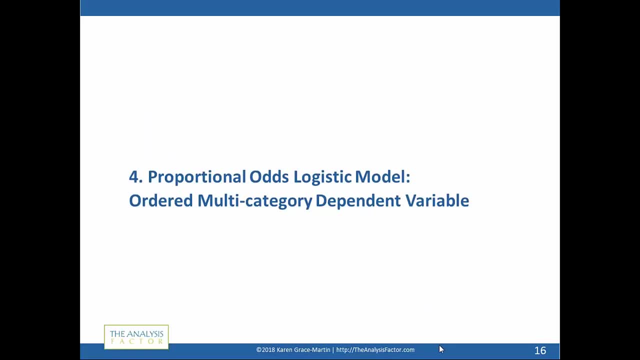 lots of flexibility, lots of information, but it can get a little overwhelming. Okay, It's a little bit different. It's a different way of expanding that binary logistic regression model when the categories are ordered. Now, before we even start, I want to mention 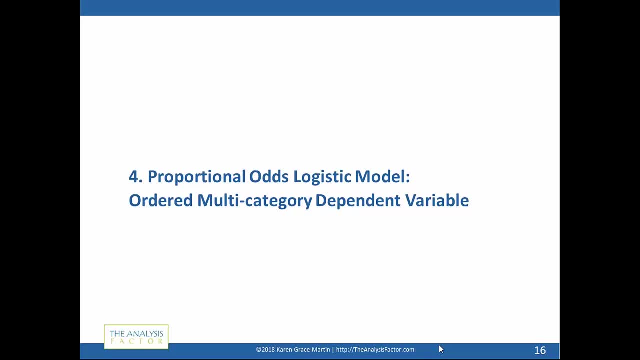 there are multiple ways of setting up an ordinal logistic regression model. We are going to talk about just one of them. It's called the proportional odds model. It is the one that is most commonly available in most statistical software. Stata seems to be the one. 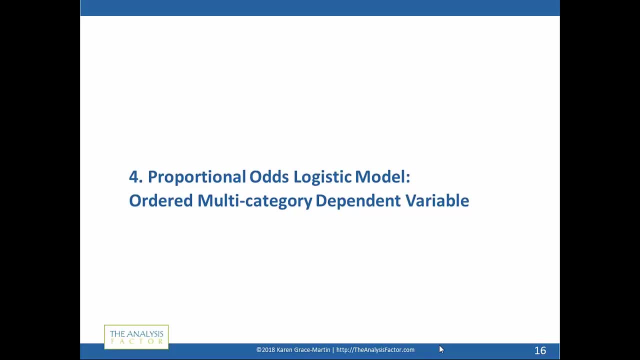 that has the most options. but if you're not using Stata, you're probably using a proportional odds model, And you'll see why it's called that in just a moment. So here and again, we might want to think about the categories differently. 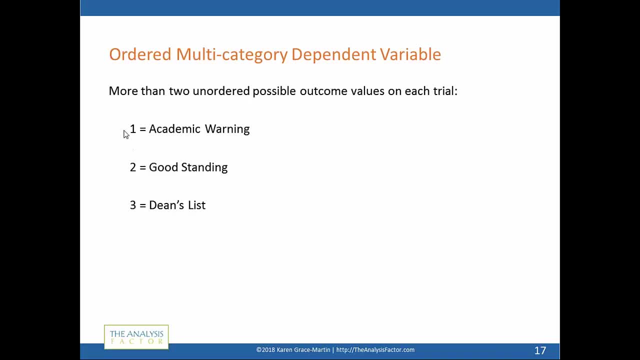 these outcome categories. So once again we might have maybe. we don't care about staying or leaving, We do still care about academic warning And then good standing. these are the students who they passed all their classes. they're doing fine. 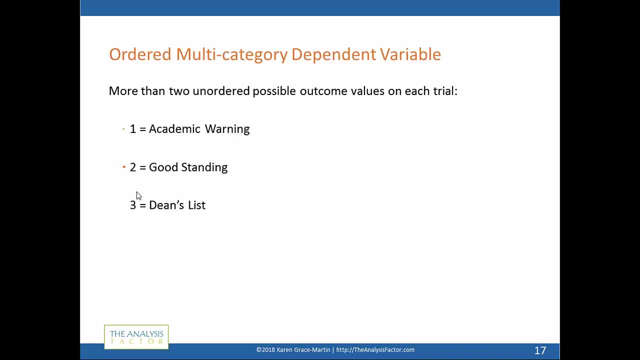 but they're not doing amazing. Okay, That's the third group. So these are the students who are really killing it. They have really high GPAs. That's the Dean's List And maybe, that's maybe- it's important for us. 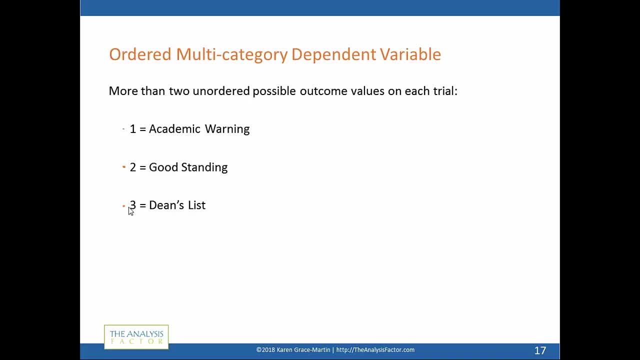 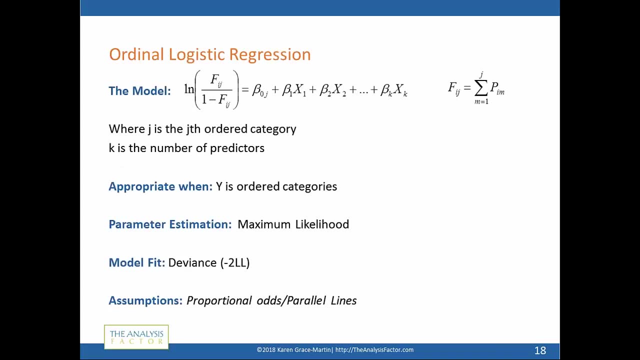 to not just see are they failing or passing, but are they failing, passing or doing extraordinarily well. Okay, so once again, it's not looking too different, but it is looking different. So let's look again over here on the right. 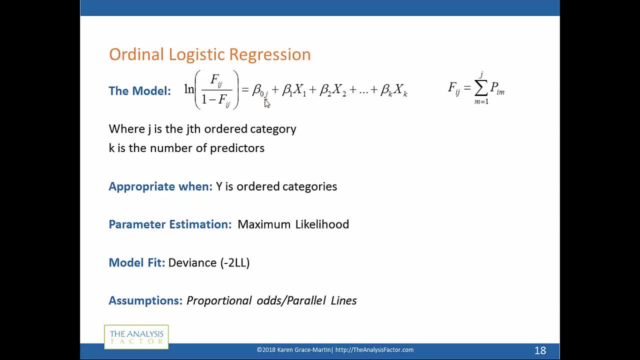 We still have this. now. we have J over here, right? So this J is the J-th ordered category. The intercept has a J, but none of the other betas do, And that's intentional, and you'll see why in just a moment. 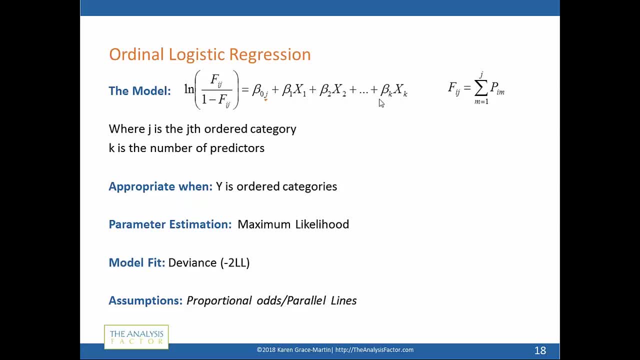 We'll jump into that, But beyond that, everything looks just like the binary case on the right-hand side. On the left-hand side, we've set up our odds ratio differently, And this particular model does what's called accumulative odds. Okay, and that's what. 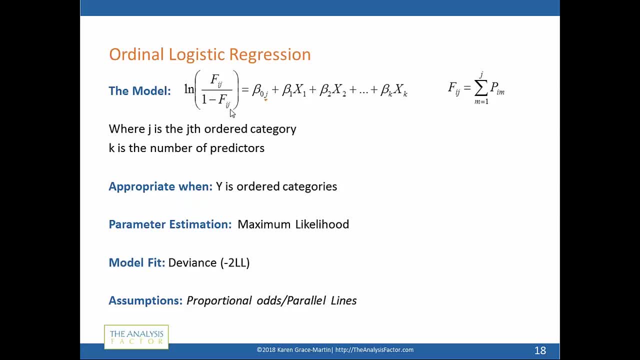 the link function is called is the cumulative odds, The cumulative odds link function. And what you will see- and there are lots of subscripts here- and it gets very confusing, and I've written it out for you on the next slide. 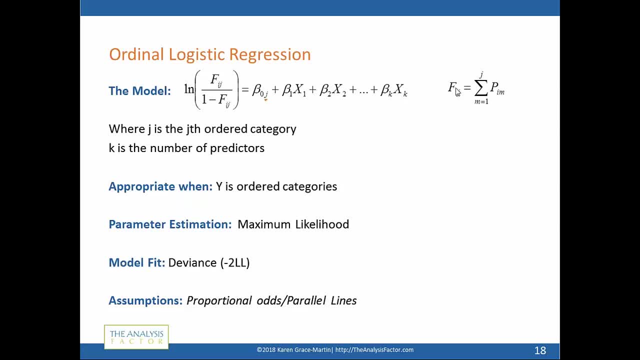 We'll take a look in just a moment, But what we're doing is F. we use F instead of P. I don't know why, but we do. But it's the cumulative probability of being in any category compared to all higher ordered categories. 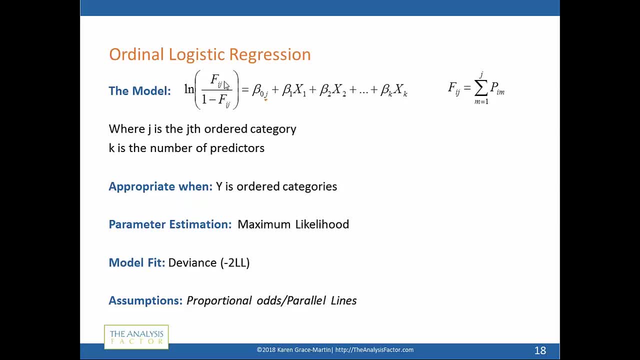 So being in category one compared to everything higher than category one, Being in one or two compared to three, and so on. So we need to have more than two categories to have order at all right. So we're going to use this when we have. 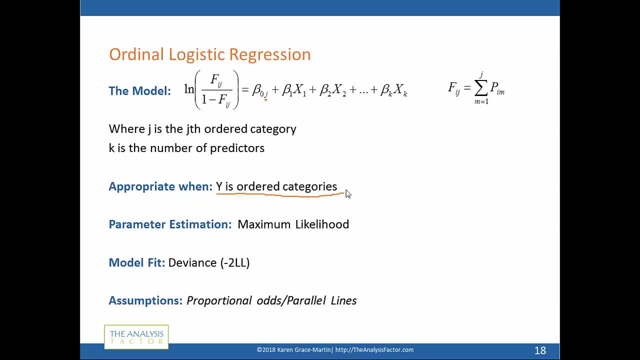 three or more categories, but they absolutely must be in order. Okay, They don't have to be equally spaced, but they have to be in order. Once again, not surprising. we're using maximum likelihood. we use deviance for model fit. 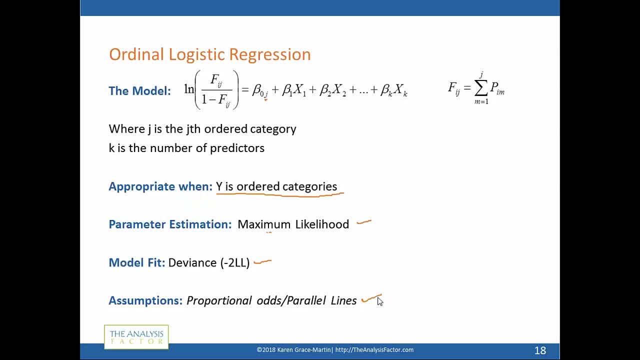 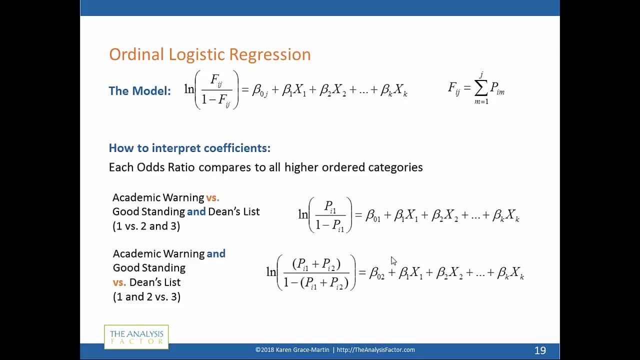 There's this key assumption called the proportional odds. Okay, And we're going to talk about that in just a moment- It's really important and it's often not met, Okay, so this whole idea of the cumulative odds is what we're doing is, again, we've got. 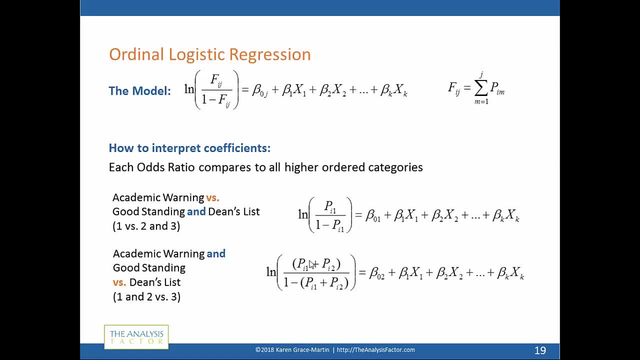 two different models, and one is looking at the lowest category- just academic warning- compared to the other two higher categories. Okay, So we've got one versus two and three. so that's why we have one and not one here. And then the 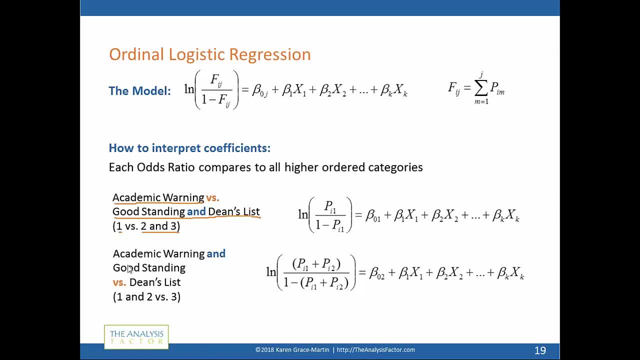 second one, we're estimating one where we're comparing the probability of academic warning and good standing, Both groups together being in either group versus being in the highest category. So one versus two and three, And this is how we're accounting for the ordering. 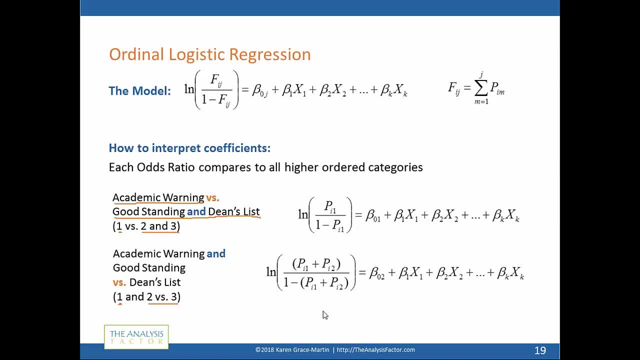 Okay, Now here's the proportional odds assumption. You will see that the intercept is different in these two models. They each have a unique subscript And this intercept, basically what it's accounting for, is the fact that just baseline values of how many people 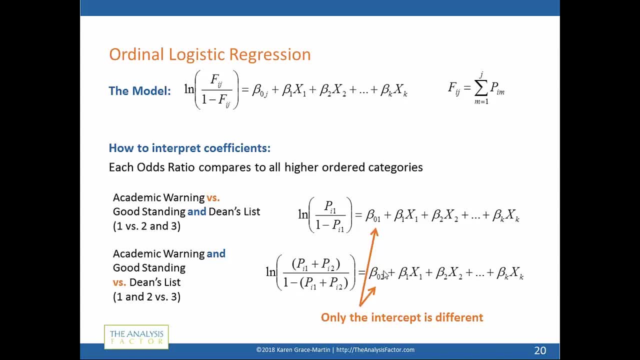 are in each category might be different. Maybe 80% of our sample is in the good standing and we only have 15% in academic warning and 5% on Dean's List. So there's an inherent different probability of being in any given. 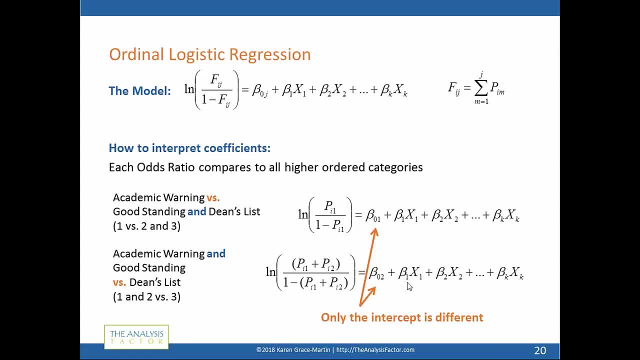 category, above and beyond the effect of any X's. But the effect of any predictor, like SAT math, on the probability of being here versus here versus there, has to be the same as the effect of SAT math on moving from one to two and three. So the 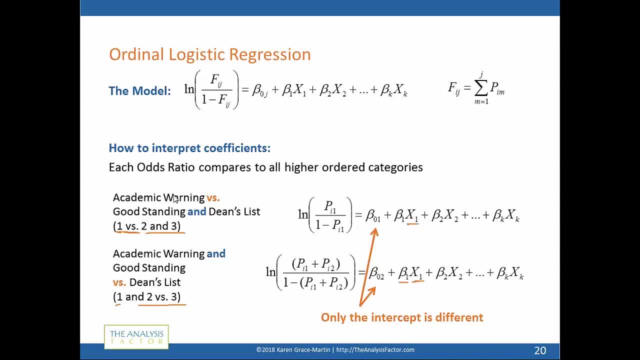 idea is the probability of being in one category versus anything higher up, no matter where you're starting along, that set of ordered categories X's affect those odds of moving into different groups the same. That's the proportional odds assumption. It is weird. 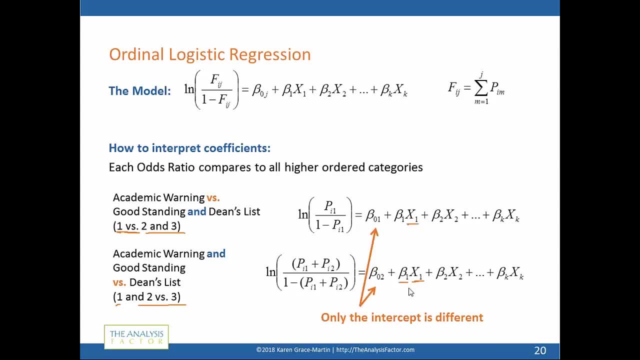 it's weird. it's totally weird and it's rarely met in data. It's pretty rare that data sets fit this Chris is asking. he gets why one is versus two and three, but why is it one and two versus three and not just two? 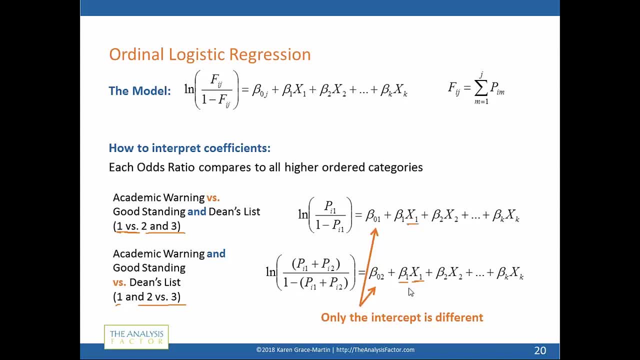 versus three. It's this cumulative probability of being in one and two versus three, and not just two versus three. It's the sum. it's the way this is set up. There is a different kind of ordinal logistic model, called the adjacent categories model. 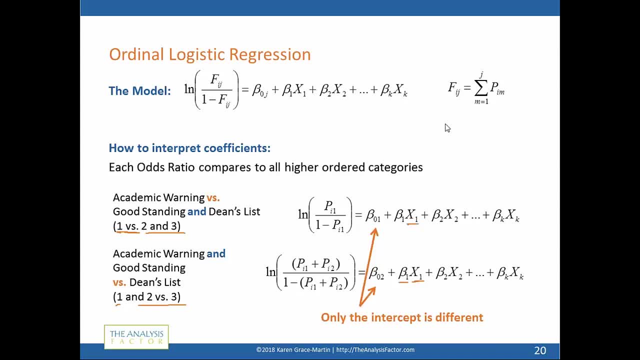 where it does that It's just looking at the next. Yes, a couple people are asking: this condition is difficult to meet, but you can test it. I have found personally it's more likely to be met when there are fewer categories. 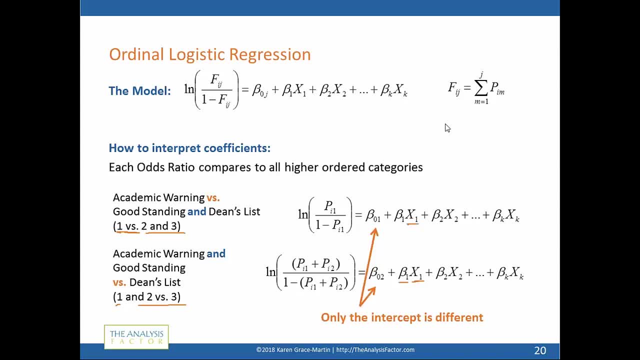 So if there are only three ordered categories, it's not as hard to meet as when there are eight. And yes, I have looked at data sets, analyzed data sets- where we have eight ordered categories. on the outcome, Does it make more sense to compare? 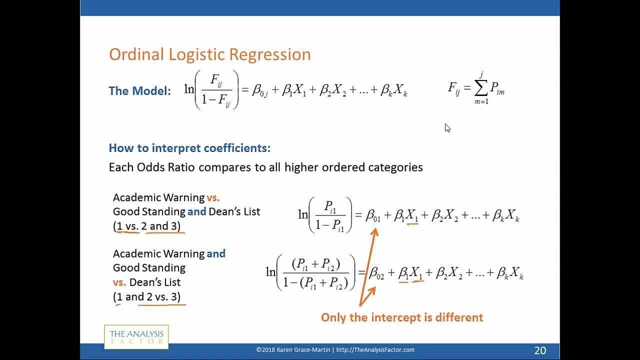 one versus two, one versus three and so on. We could do that by running the multinomial model, the unordered one. There are tests, There are tests on this assumption and really the only way to truly tell if you've got this is to: 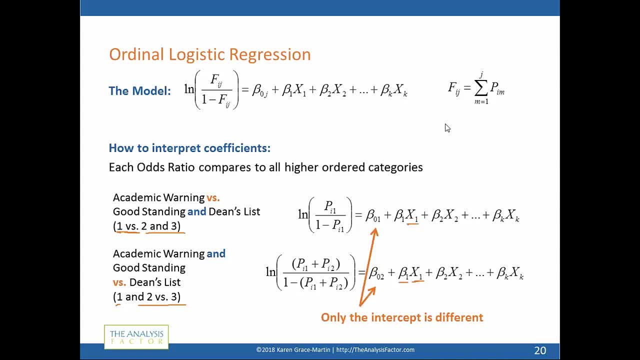 run one of the other models. There is something called a generalized ordered logistic regression that uses the same link function, but it does not force these betas to be equal, And that's the one that Stata has a very nice function called GoLogic2. 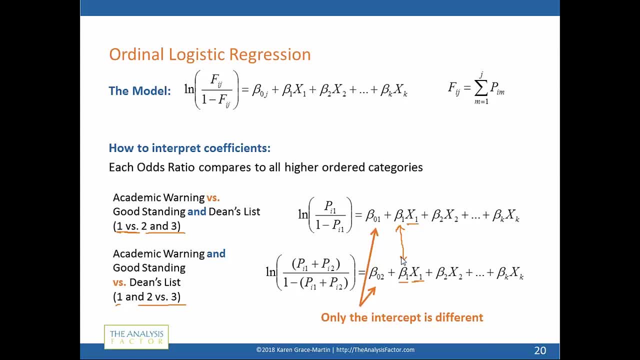 that does that for you automatically. Okay, so we have about seven minutes left. I do want to take a few minutes to answer questions. I am sure I will not get through all the questions. We have right now about 300 people here, but 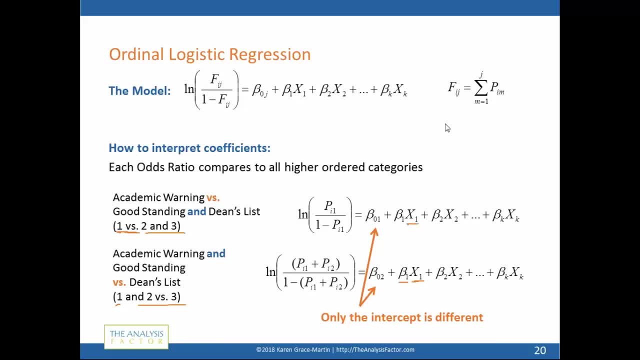 we can download all these questions and save them and we'll answer them on the website. So please ask, even if we don't have time to get to your question. How do we measure model fit with deviance in comparison to AIC and BIC? 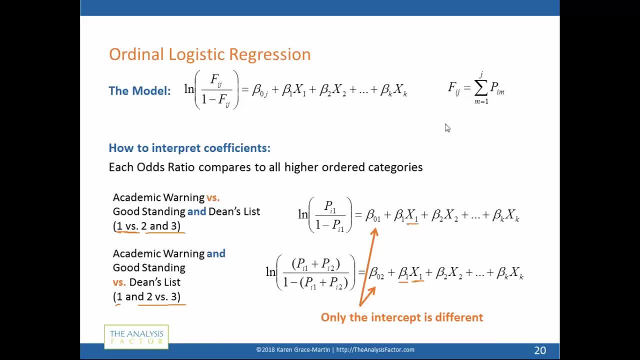 Which is better and why. Okay, AIC and BIC are based on the deviance statistic They have. it's not that one's better or worse. They have different advantages and disadvantages. So deviance you can actually get a p-value for. 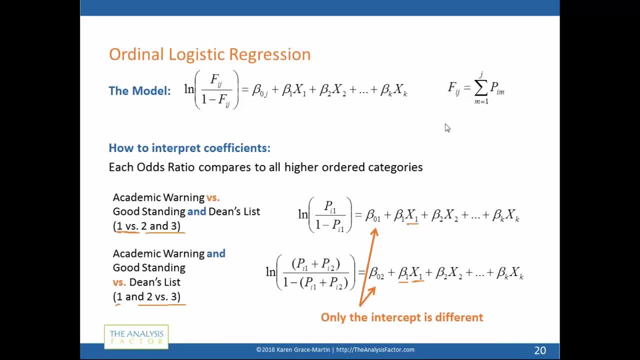 So you can actually compare two models, get a deviance statistic for each one and see if one model is, you know, actually get a test whether one fits better than the other model. But models have to be nested, Meaning one has to be a pure subset. 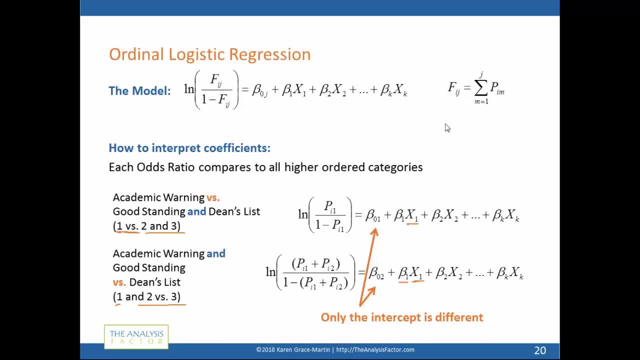 of the other, So it's a bit restricted. AIC and BIC don't have the p-value but they also don't have the restriction of being nested models. Good question Juan asks: can we run a sort of sensitivity analysis to compare models from? 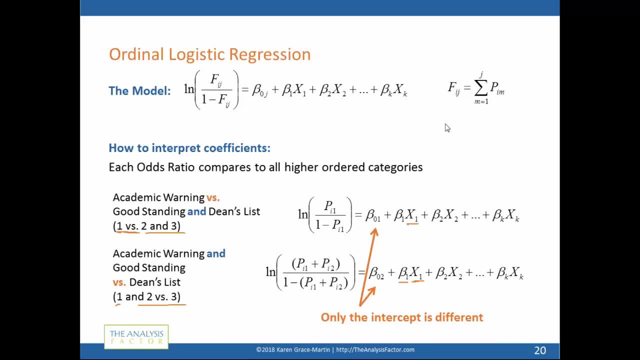 multinomial versus ordered if the assumption of proportionality is met. I don't know if there's an official sensitivity analysis where you can do that. Certainly in the GoLogic2 it will still do the same link function that the cumulative link function on both. 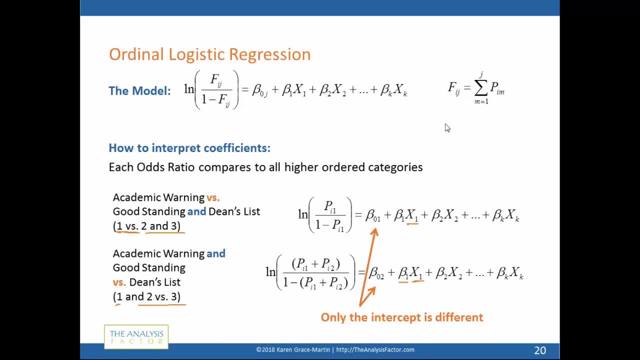 but one constrains the parameter estimates to be equal and the other doesn't, So you can do it there. But if you're truly doing a multinomial model versus the ordinal, then it's a little bit different because you're actually using a different link function. 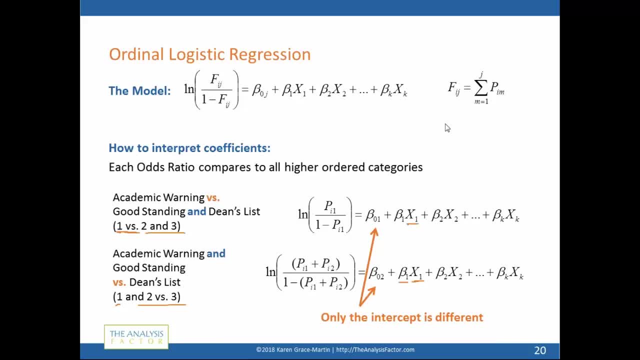 You're comparing the odds to different groups, So it's really they're not comparable. Oh, Jerry has a great question. What about the Nagelkirche R squared? First of all, let me say I have no idea how to pronounce that person's name. 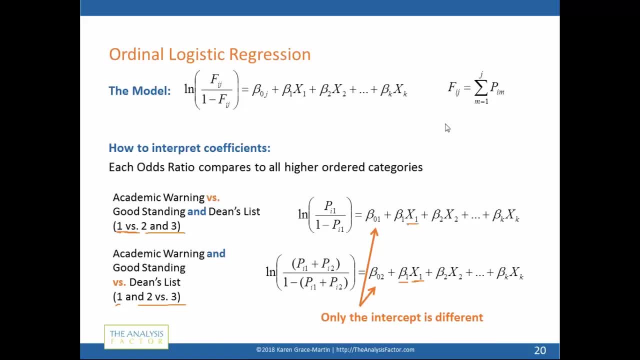 There are a number of pseudo R squared, including that one available usually on your software output. They do not have that same interpretation that we get from a regular R squared, so it's not percent variance accounted for. They do. there are different versions of it, if I 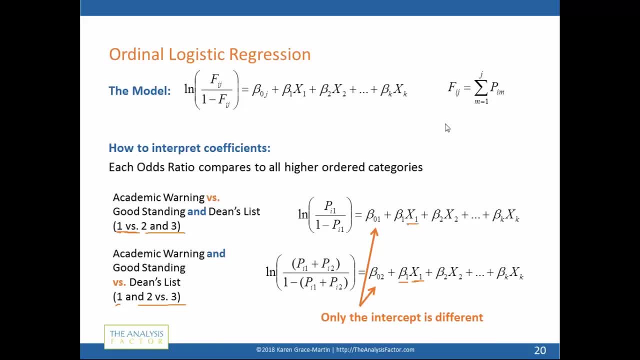 recall correctly, the Nagelkirche can never equal one, So the top possible value is lower than one. So there's an adjust. somebody else has an adjustment to it where it can go all the way from zero to one, But in general you tend to get. 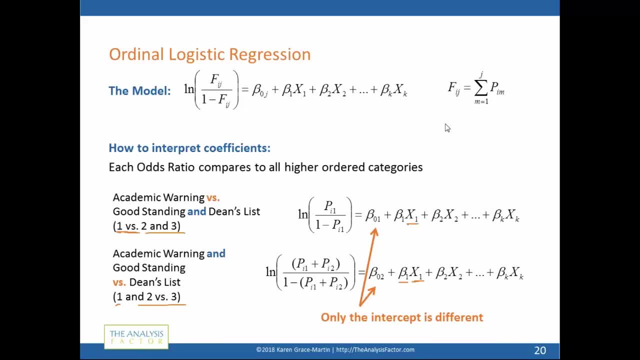 lower values on those pseudo R squares than you do in, say, a linear model. So they tend to look terrible, but it's just the nature of them And like the highest one I've ever seen in a real data set is something like 0.19. 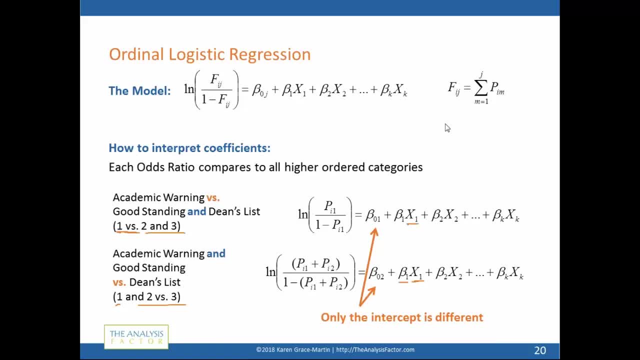 they're really quite low And they don't have that nice interpretation. So they're there, but they're not as useful as we'd like. Ah, okay, Doug has a great question. In the binary model you can get a probability of being one and probability of being. 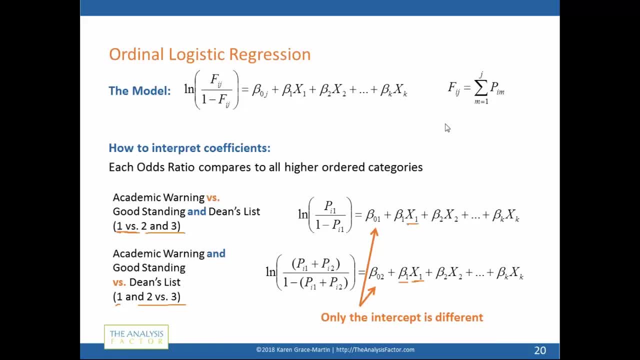 zero In a multinomial and proportional odds. can you arrive at the probability of being in category? oops, it just scrolled down. I think it was one, two and three. You can. It's a little bit more work, okay, because 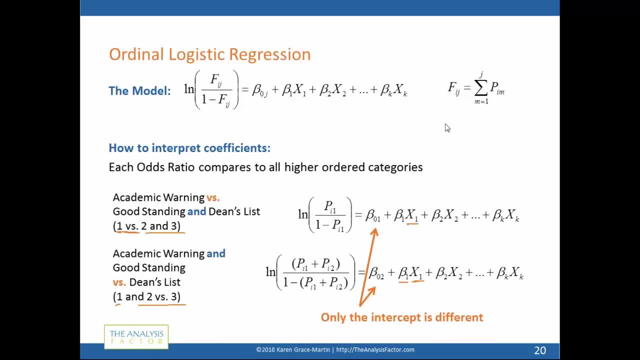 what you have. you can get predictive probabilities for each one. They are not intuitive. This is something we do in the workshop. I show you how to get each one. Sometimes, what you have to do is figure out what's the probability of not two. 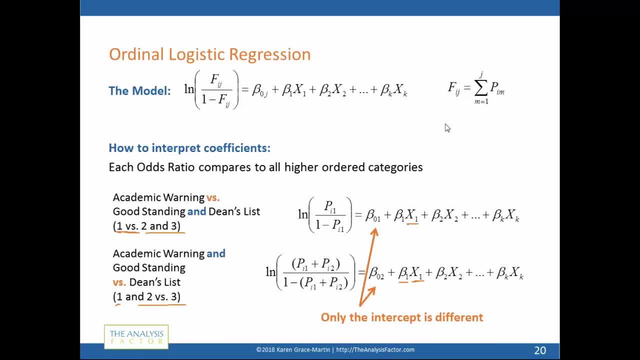 And from that take one minus that probability to get the probability of two. So it's a little bit more finagling, but it does exist. Jesse asks: is there a good way to graph these results? Yeah, usually you graph it through either predicted odds. 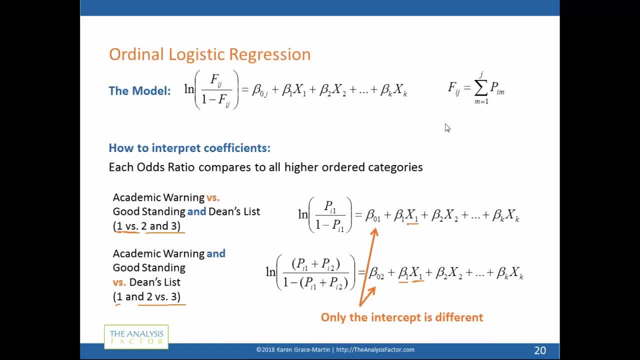 or predicted probabilities. Predictive probabilities are a little bit more intuitive to people, But it's also you have to be a little bit careful there, because it's so, for example. let me give you an example. Let's say you're drawing predictive probabilities. let's say you have